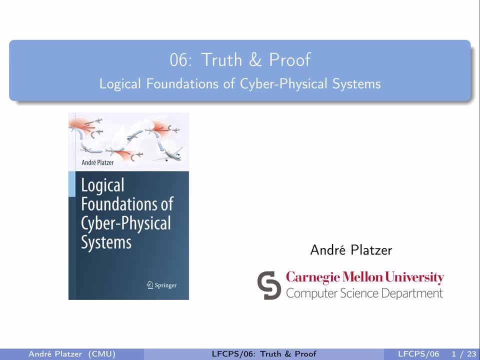 as long as we exactly knew how to use them. That's where the question for today comes from: How do you best tie the individual inferences together to obtain a well-structured proof? In fact, what is a proof? to begin with? It turns out there's much more to proofs than 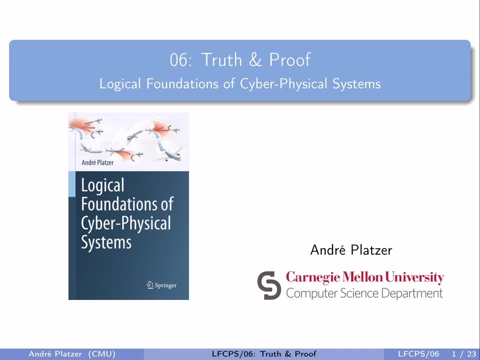 just axioms, There's also proof rules that are meant for combining fragments of arguments together into a bigger proof. In other words, proofs are the glue that holds axioms together into a single cohesive argument for which you justify the conclusion of the proof. 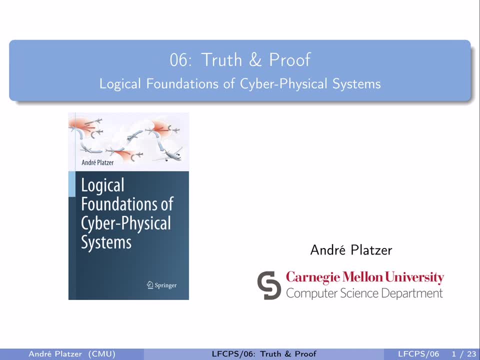 For example, when we were proving quantum, the acrophobic bouncing ball- okay, admittedly, single hop, but never your mind- we seemingly applied axioms at random at all kinds of places in the formulas and then call it a day. That's fine when you look back at such a proof and 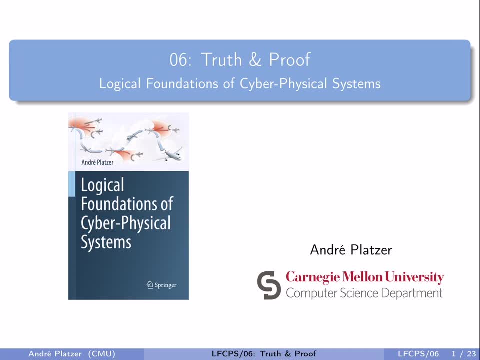 appreciate how elegant and simple and beautiful it was, but it's not so helpful if you're trying to come up with such a quote, unquote, random proof in the first place. More guidance is helpful. Another part where we've been very informal is how to justify. 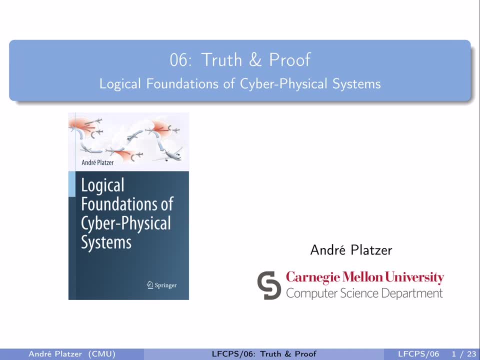 the resulting arithmetic, which, if we continue to be informal about that, leaves plenty of room for subtle mistakes and correctness arguments. We should never have subtle mistakes, nor any mistakes at all when it comes to CPSs. What we will be doing today is imposing more. 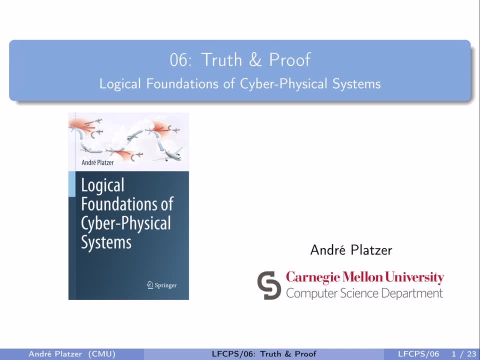 structure. on proofs, For example, We'll learn what to do with the propositional connectives such as and or implication and not, but also the first order quantifiers such as for all and exists. We haven't seen anything about them yet. 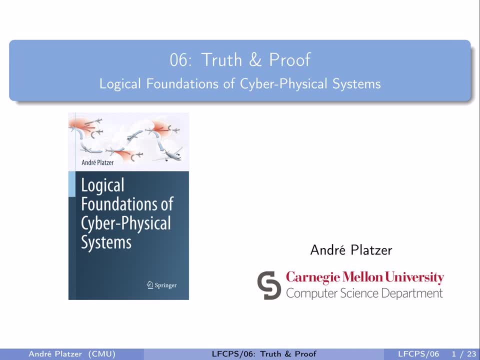 We'll also revisit the fundamental proof principles for dynamics that we saw and make them more systematic. because, well, the axioms were just that: they were axioms. That's amazing, because This is always valid, It's true, in all states, but the axioms didn't exactly tell us how. 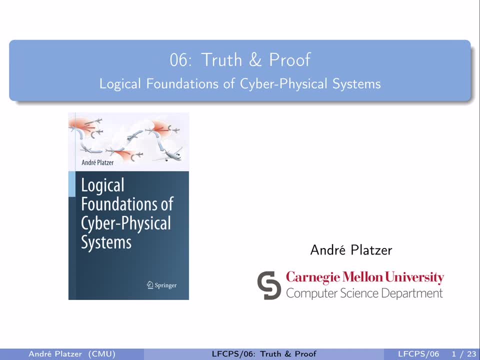 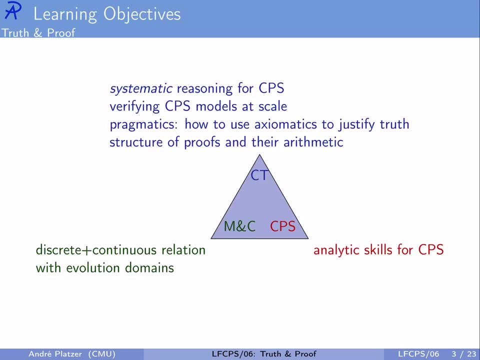 they're meant to be used in order to make sure we actually make our reasoning easier. so we'll look into this today. On the modeling and control side, we will deepen our understanding of how discrete and continuous dynamics relate, because we'll understand in more explicit, better proof-based ways. 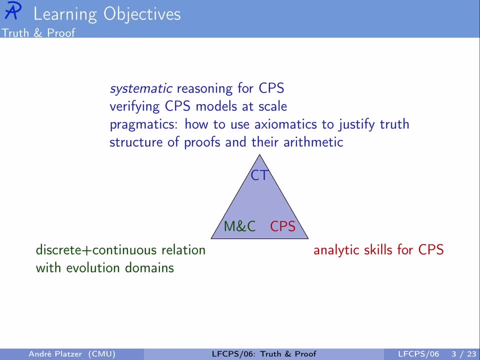 and we'll be able to do that in the next class On the proof-informed ways, how the discrete and continuous dynamics relate in the presence of evolution domain constraints, which we briefly talked about last time On the computational thinking side. today's topic is really about not just reasoning for 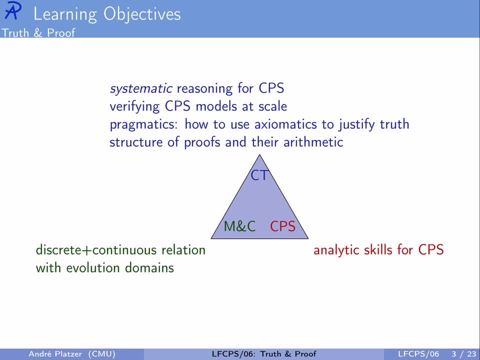 cyber-physical systems, which we saw in its beauty last time already, but also systematic reasoning for cyber-physical systems to make sure that we really know what we need to do. when we're trying to do something, We're going to develop a proof for a system, and that's, of course, completely fundamental. 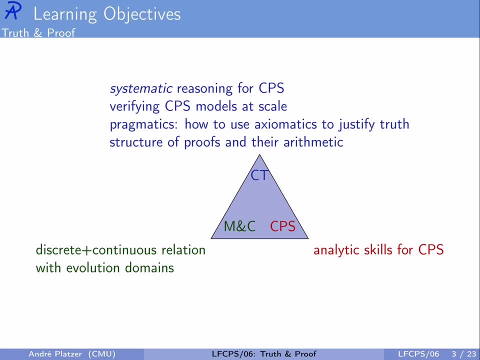 for having any chance at all of verifying cyber-physical systems models at an appropriate scale. For simple things like the bouncing balls, we could make do with what we had, but there's just no chance you're going to do the same thing for the full complexity of an aircraft. 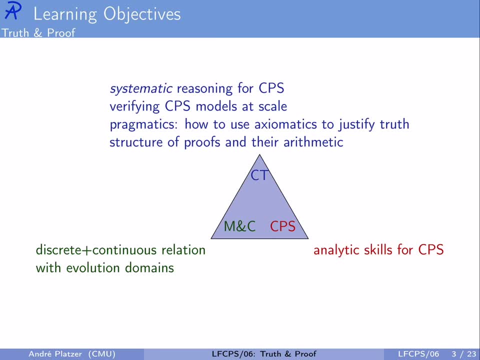 without more rigorous structuring principles. In particular, we'll discover the pragmatic aspect of proofs, by which I mean how they work, how to use the axiomatics to justify the truth of syntactic expressions. We'll also be structuring proofs and their arithmetic arguments. 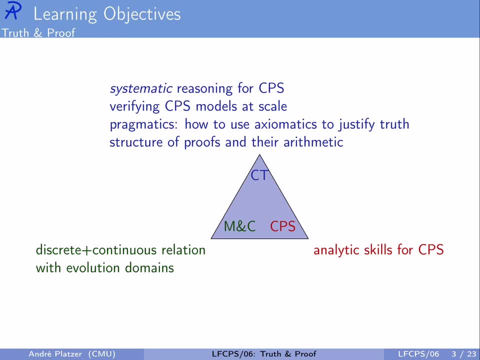 Our CPS skill side will be mostly devoted to sharpening our analytic skills for cyber-physical systems, but we will also develop a slightly better intuition for the operational effects, in particular, in terms of questions like: in what order should we worry about operational? 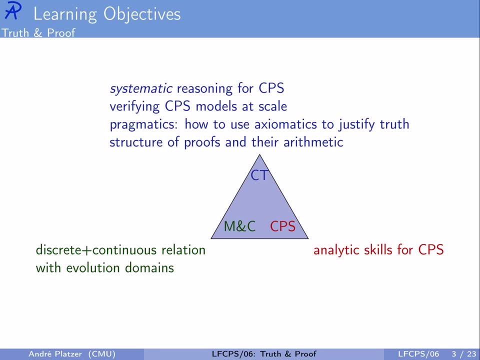 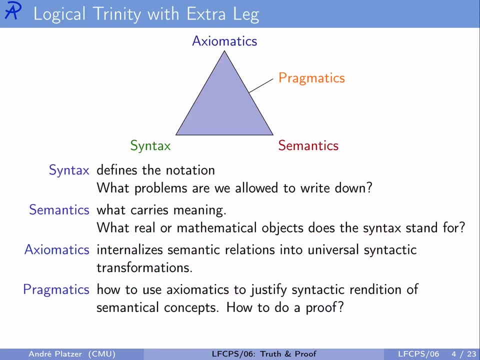 defects, In particular in terms of questions like: in what order should we worry about operational defects? In particular in terms of questions like: in what order should we worry about operational effects and does that matter? For the logical trinity that you saw today, we're essentially adding an extra lag: the 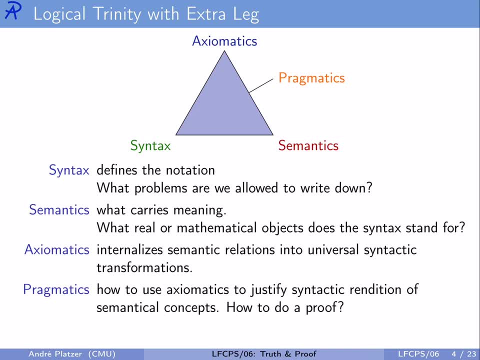 pragmatics, by which I mean, in addition to the syntax, which is just defining the notation for the problems, we can ask the semantics, which is defining what actually carries meaning. What's the real or mathematical object that we're talking about? 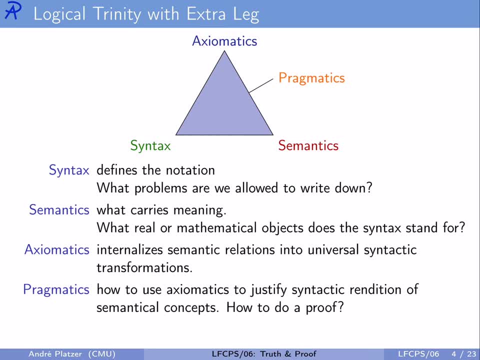 The axiomatics we saw last time, The axiomatics we saw last time- which internalizes the semantic relations between objects as universally useful syntactic transformations. Just think of the axioms. We had a logical syntactic axiom which once and for all, taught us that two logical formulas 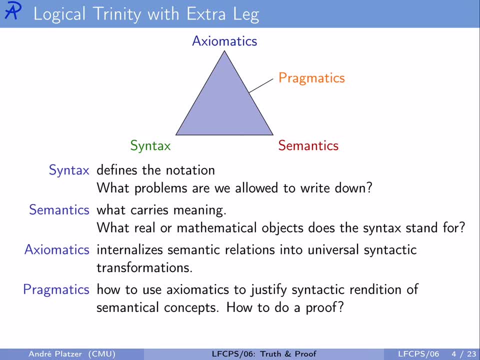 are always equivalent, so we can swap out one for the other in any hard place. But none of what we saw so far told us how to pragmatically go about using the axiomatics to justify the syntactic transformations, quantify the syntactic rendition of semantic constructs. How do we even do a proof in the 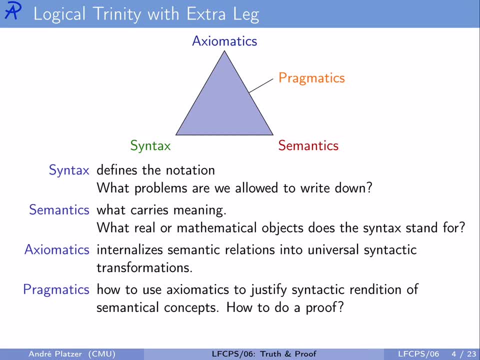 first place, In what order do we proceed? The axioms? well, they were equivalent axioms. They equated the truth of two logical formulas with one another. but should we use them from left to right, or should we use them from right to left? What makes things easier? Each of? 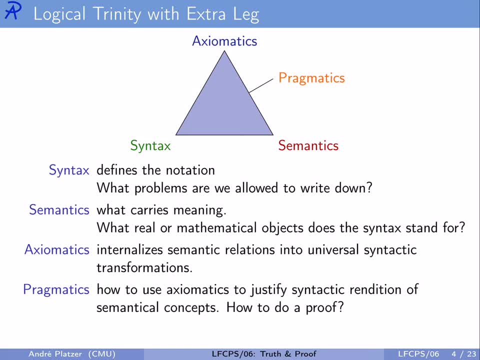 the axioms was an equivalence which equates the true values of two differential dynamic logic formulas. but how are we supposed to use that? It's an equivalence, all right, It has two sides. Is the left-hand side nicer? Is the right-hand side nicer? Should we use? 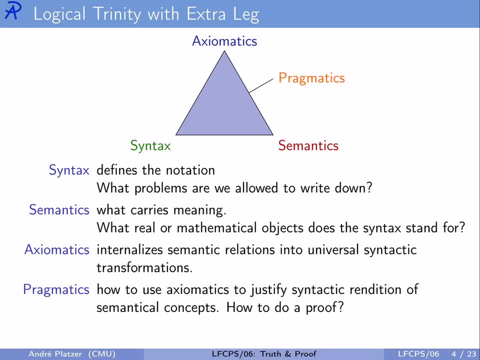 it to transform the left-hand side to the right-hand side? Should we always use the backwards direction? Should we use one of the implications, In other words, this pragmatics of how to go about doing proof search is one of the important concepts of proof search. 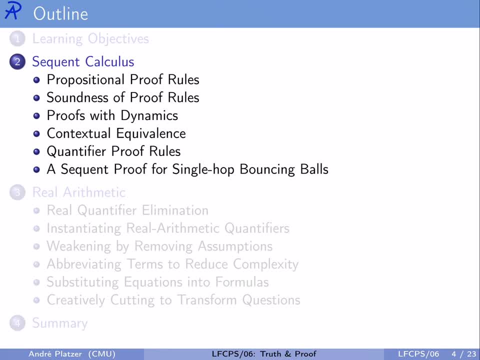 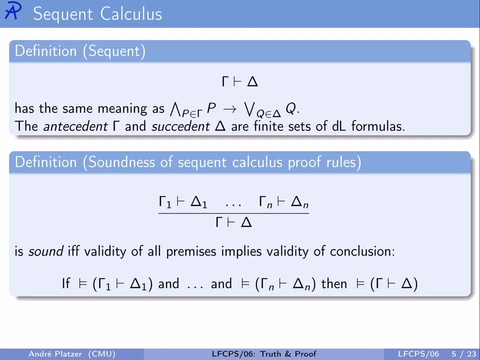 For that we will be looking at an extension of Gerhard Gensson's sequent calculus, which is basically a way of making proofs and arguments completely systematic. Sequence are these constructs for a finite set of formulas gamma and a finite set of formulas delta, The gammas? 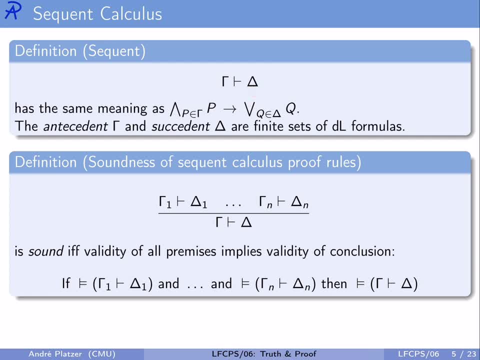 are called antecedent. The deltas are called antecedent. This sequent is just a way of normalizing what we know. Gamma you should think of as all the assumptions that we have available for our argument at this moment, and deltas you should think of as all the alternatives that we're trying to prove. We're not trying. 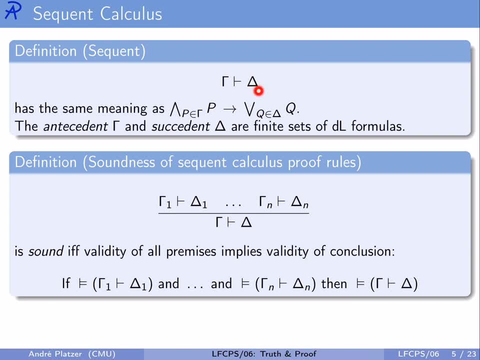 to establish all of them. We're just merely trying to establish one of them, In other words a sequent gamma turn-style. delta is just an abbreviation for this logical formula that says the conjunction of all the formulas on the left-hand side, the antecedent. 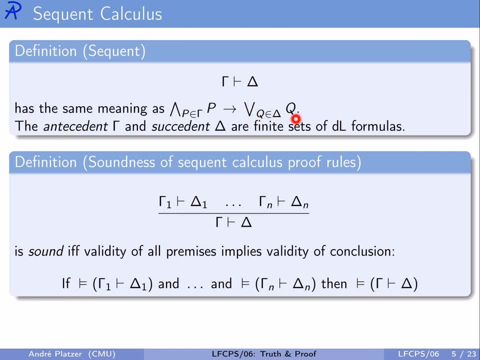 implies the disjunction of all the formulas on the right-hand side, the succident. Think of it this way: In the antecedent gamma, you may have assumptions such as: the moon is a ball and the moon is big In delta. you may have a list of options you're trying to prove from that, For example, the 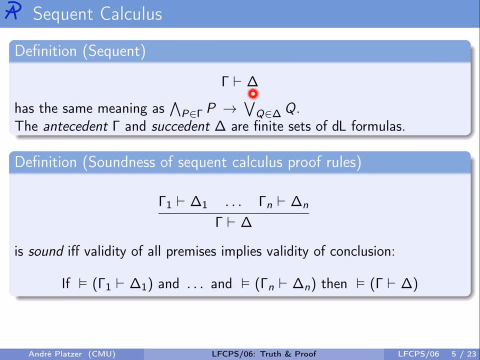 moon is round or the moon is a square. Now, you certainly wouldn't be able to prove both of those- that the moon is round and the moon is a square- from these assumptions. but one of them will do from the assumption that the moon is big and the moon is a ball, because 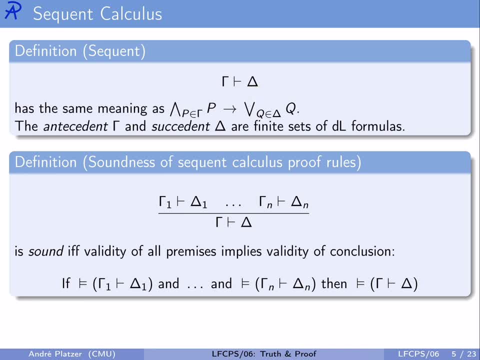 balls tend to be pretty round. In other words, the deltas are the options that we still have available for proving in our arguments, and the gammas capture all the assumptions we presently have Now as a sequent. what we do in a proof, in sequent calculus, is to systematically 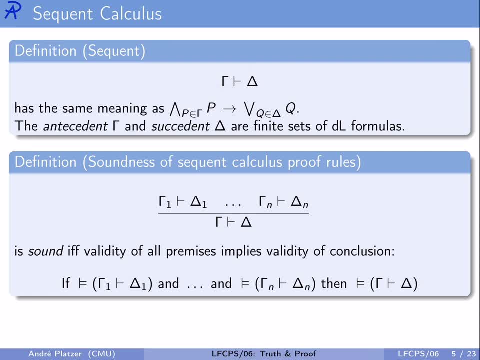 transform one sequent into other sequents using sequent calculus proof rules. The sequent calculus proof rules all have the shape that for some number n of premises they have a sequent as the first premise and so on, and the sequent as the nth premise From these premises. a. 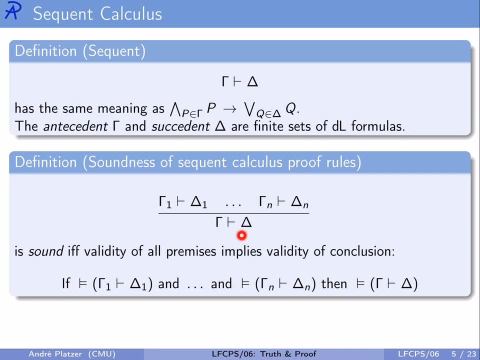 sequent calculus proof rule is concluding a sequent. that is the conclusion. We use these sequent calculus proof rules in an admittedly weird but historically logical way. bottom up, That means we reduce the question whether this sequent has a proof using this proof. 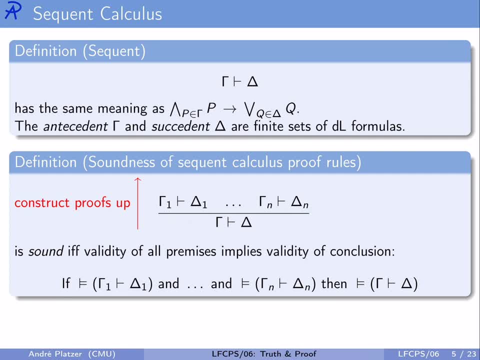 rule here. I write with this bar notation or inference rule to these subquestions or subgoals whether this sequent has a proof, and so on, and whether those sequences have a proof. The idea is that, in order to answer whether this sequent can be proved, I will instead ask myself whether 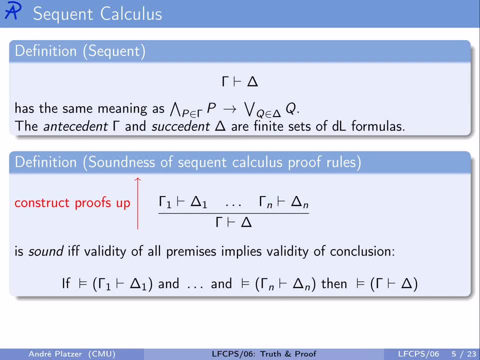 this and that one can be proved Having done so. if I've succeeded with a proof of this and so on and the proof of that, Then we come back in our argument to make sure that if this has a proof and so on, and these have a proof, that means if all the proof 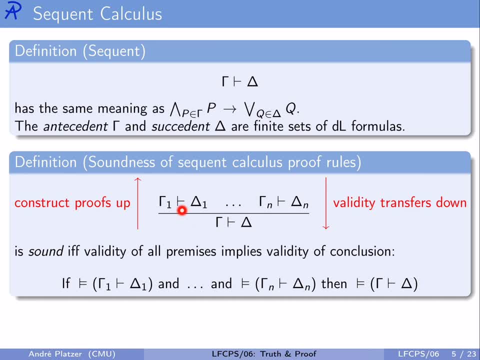 rules we used are sound, that these sequence all represent, by this encoding valid differential lemma logic formulas. That means that if all of these have proofs or they're valid, then that sequence also has a proof, So it's valid, which, of course, is only the case if we don't. 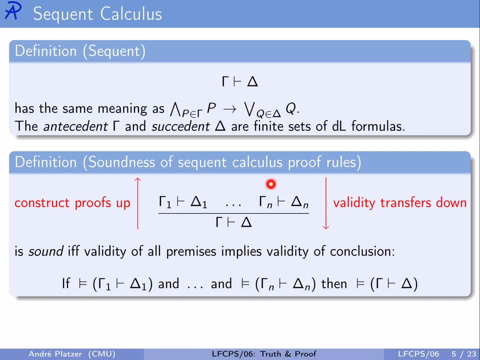 use an arbitrary transformation as a sequence calculus proof rule, but only sound ones, The ones that say: if all the premises are valid, so they're true in all states, then the conclusion is valid, so true in all states. Wait, wait. 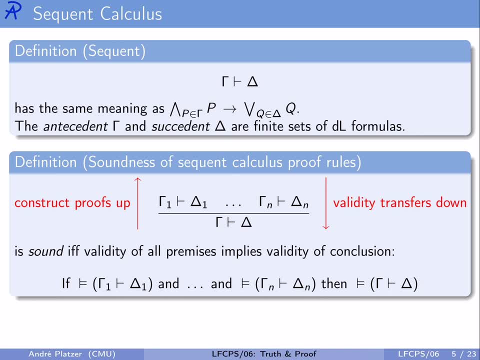 When is this sequence valid? Well, that's actually already defined. Look at this one, for example: Gamma turns to L-delta is actually just a syntactic representation or a normal form for a differential lemma. logic formula of this shape. Conjunction of every formula. 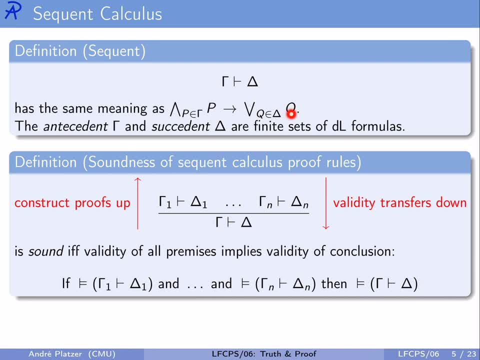 on the left-hand side implies disjunction of all the formulas on the right-hand side For a differential lemma logic formula. of course we already said, when it's valid, it's valid if it's true in all states. So what we need to do now 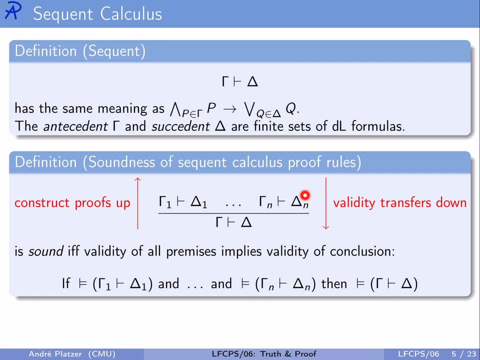 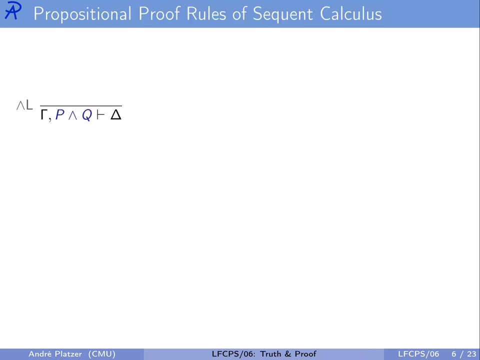 for example, is develop specific proof rules. We'll still use logical compositionality arguments as guiding principles to develop one proof rule for each operator or one proof rule for each shape that the formulas within gamma and within delta can have. Let's do just that. 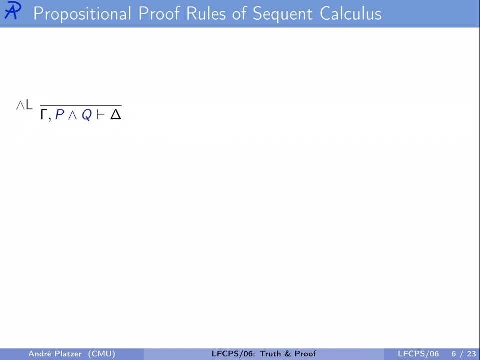 For example, we would need a proof rule that is called and-left For handling and operators, so conjunctions on the left-hand side, so in the intercedent. What does that mean? That means we're asking ourselves how do we prove a sequent that 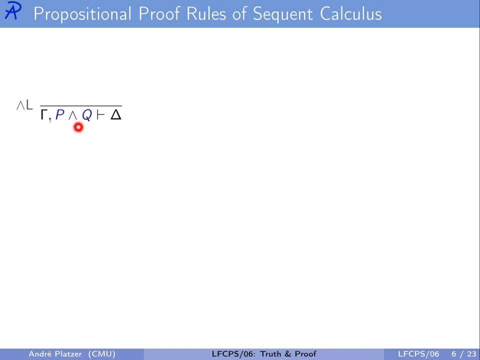 says: we've got some assumptions gamma and an assumption P and Q and we're trying to prove delta from that. Well, what do you do? if you are assuming a conjunction P and Q? How can you say that in delta Logically simpler, smaller ways? Well, assuming P and Q is, of course, the same as assuming. 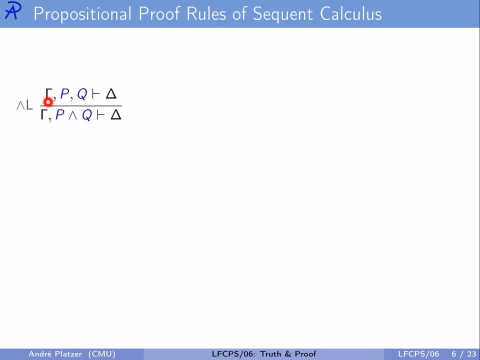 P as well as assuming Q in addition to the assumptions you already had, Then still proving the same question: delta from that. That means you're assuming conjuncts separately, which makes a whole lot of sense, because if you're assuming that P and Q is true, you might as 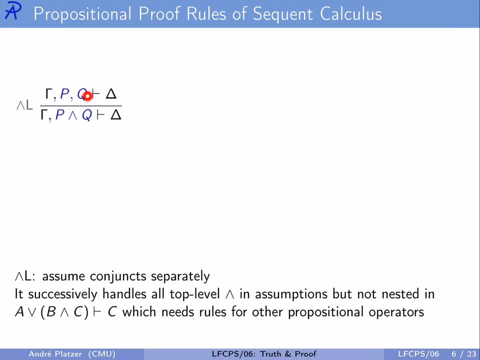 well, assume that P is true and also assume that Q is true. If you now keep on using the and-left proof rule that you see here on the slide for all the top-level and operators of all the formulas that appear in the intercedent. the top-level: 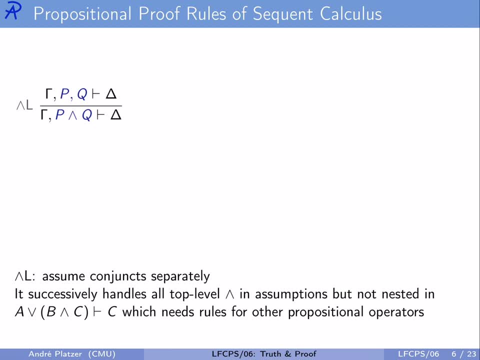 and the proof rule will be able to handle and simplify syntactically each and every one of them. Okay, Also, if a conjunctive formula- P and Q- occurs within gamma, because if this is a list of formulas or a set of formulas, because it doesn't make a whole lot of sense to assume. 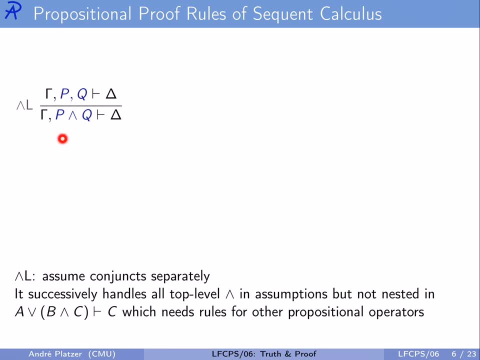 the same thing twice, then we're implicitly able to always use the proof rule, no matter what particular position it occurs in the antecedent. We're not allowed to use the same proof rule just because it occurs in the things we're talking about. 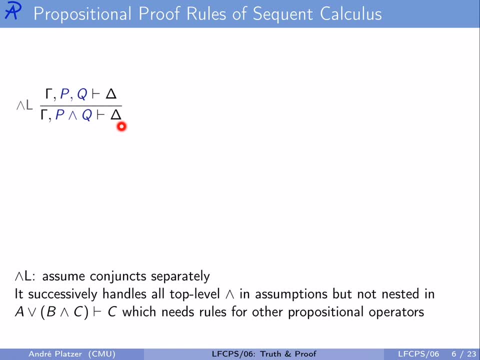 We're not allowed to use the same proof rule just because it occurs in the things we're trying to prove from that, because that might be a different logical reasoning principle But for example, that can handle all kinds of situations, not this one. Because if our 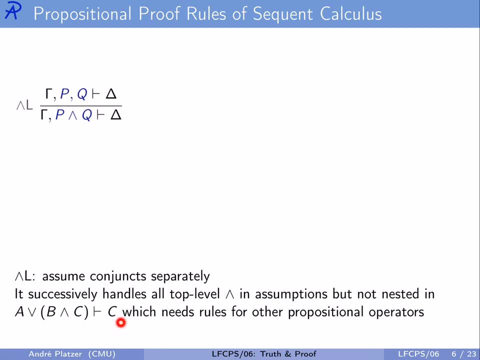 sequence is A or B and C and from that we're trying to prove C. whether or not that will succeed is another question. but even if there is an and in it, it's not on the top-level of a formula in the antecedent, because the top-level operator here is an or, which means 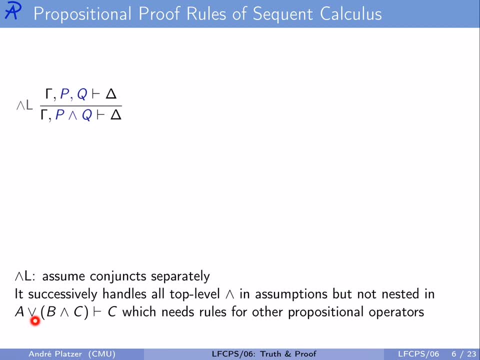 at some point we need to worry about the antecedent. Wait, how do we prove? or assumptions on the left-hand side? But first let's ask ourselves: how would we if an and occurs on the right-hand side in the seccedent? how would we prove? 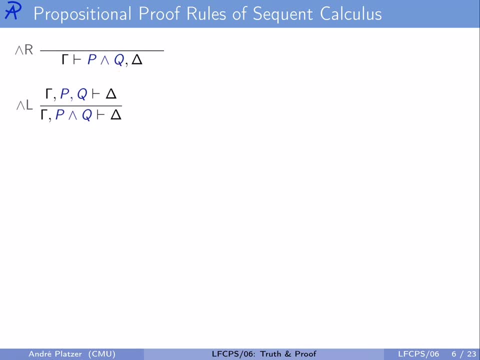 that P and Q is true. What would you do as a mathematician? Well, to program a bunch of assumptions- gamma- you would prove that P and Q is true. ignore the deltas for now. by proving that P and Q are true, You would prove that P and Q are true. ignore the deltas for now, by proving that P and Q are true. 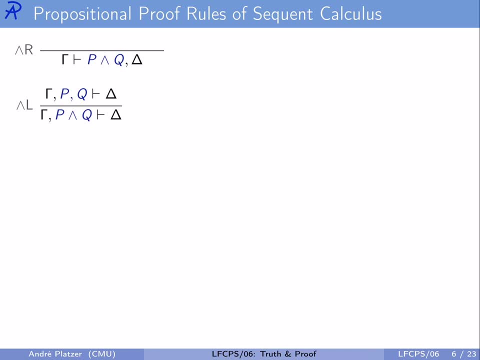 You would prove that P and Q are true. ignore the deltas for now. by proving that P and Q are true from the exact same assumptions- gamma- and by proving that also Q is true from the exact same assumptions, You would be proving this sequent and, having done so, also prove the average sequent. 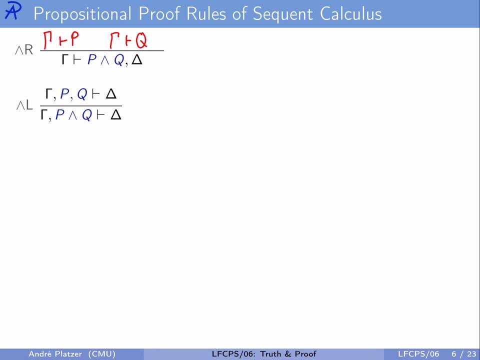 Now, what's with the delta alternatives that we could be proving as well? Well, here we're not actually trying to prove just P and Q, We're trying to prove P and Q or any of the alternatives. really, If we succeed with the proof of P and we succeed with the proof of 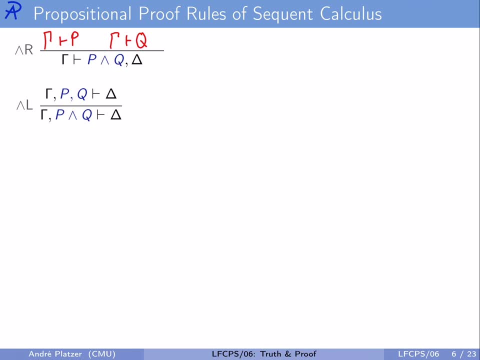 Q. that's fine, We've proved P and Q or some other nonsense. But suppose we're succeeding with this proof only because we established a proof of the other nonsense. Well, in that case, if we prove this other nonsense, delta, everything, all the other alternatives in. 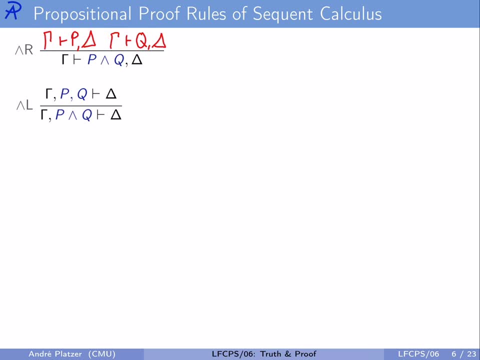 this sub-question and in that sub-question then of course, we've established a proof of that. In other words, proving conjunctions is what we would do by proving each of the conjuncts separately. Proving that P and Q is true requires a proof of P and a proof. 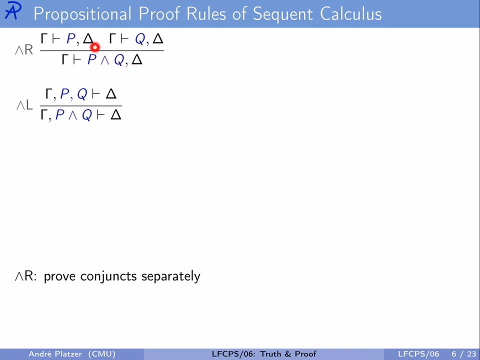 of Q, but we will keep all the other alternatives. We'll keep all the alternatives around, just in case the proof of those proceeds better. Now, how would we prove a disjunction Proving that P or Q holds true? well, or maybe some. 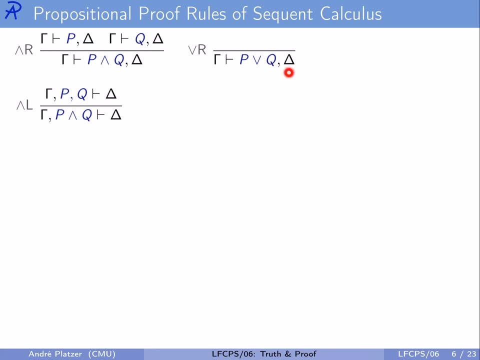 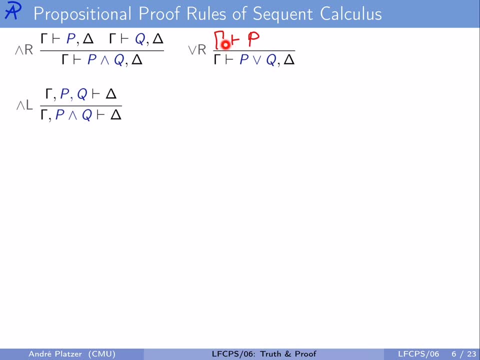 kenmer. But if we were to do that, then, just like in constructive logic, we've basically committed to one of the two sides of the disjunction and proved precisely that That will be unnecessarily complicated In our classical logic. what we will be doing instead. 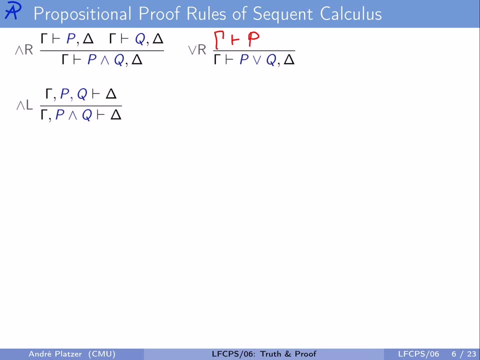 is to also accept the proof of Q instead of the proof of P, if that works. Ah, I said the magic word Okay, Okay, or In other words, what we need to do here is: it's also fine if we prove Q from that. 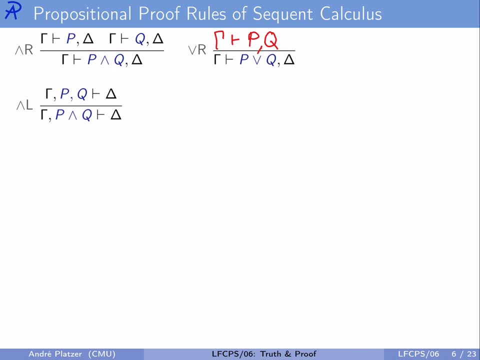 instead, and we already have something that keeps alternatives as managing whatever things we could be proving from our assumptions gamma. It's called the comma operator. Remember the meaning of a comma? on the right-hand side of a turnstile sequent is an or, whereas the 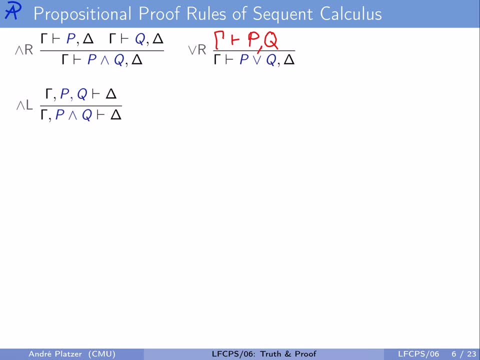 meaning of the comma on the left-hand side is an and, Of course, if we keep any of the other options and succeed in the proof of those, that also still proves the things we already asked to prove, namely to prove from the assumptions gamma that P or Q is true. 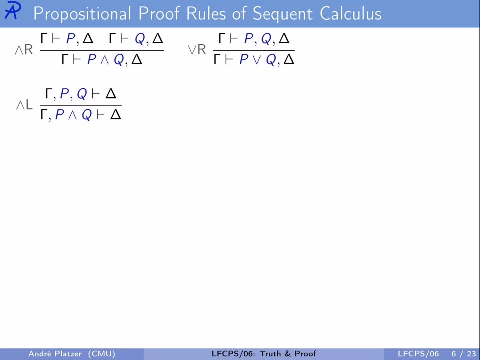 well, or the other alternatives. Our proof rule that we've got is right here. That's the proof rule for proving a disjunction by splitting the disjunction into its separate parts In the exact same succident, because the comma in the succident already has a disjunctive. 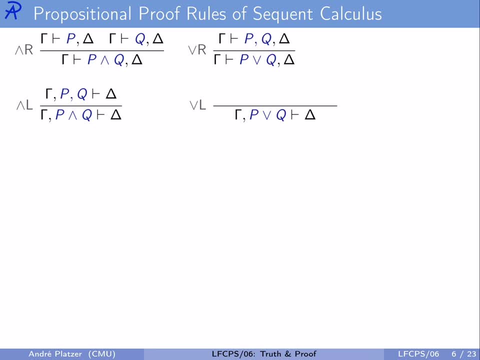 meaning. How would we then go about doing a proof in which we have a disjunction among our assumptions? Among our assumptions, we find that P or Q is true. Well, if, among other things, we assume that P or Q is true and we're trying to prove delta from that, then 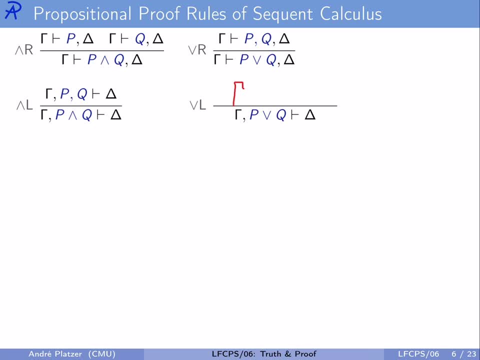 we can't exactly proceed with a proof that what we're trying to establish, delta, follows from the assumptions gamma together with P, because we don't even have P among our assumptions here. We merely have P or Q among our assumptions. We know that P is going to be true or Q is. 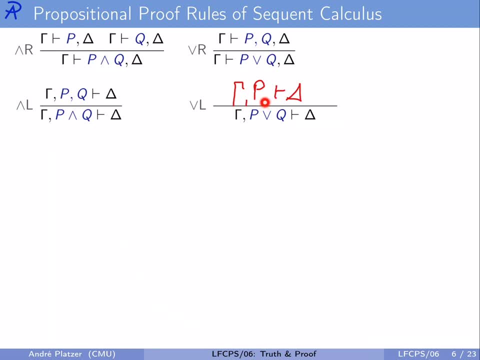 going to be true, but we can't commit to every side because we have no way of knowing. But We can do that again. We can separately show from the assumption Q instead that delta also follows. Here's the proof rule: Assuming P or Q among our assumptions and going for a. 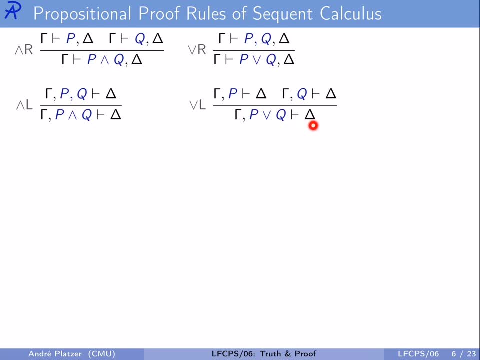 proof that this, together with other assumptions gamma, allows us to establish delta from it. for that it suffices if we prove from the assumption P and the other ones that delta works out, and also from the assumption Q and the other ones that delta works out, Because 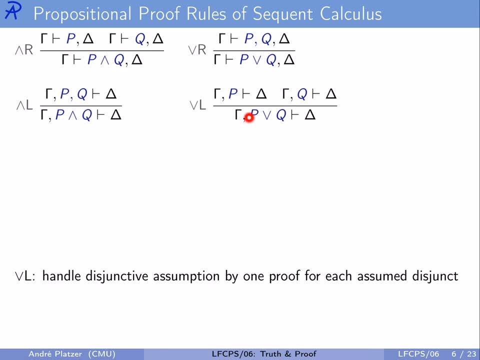 whether the assumption P or Q was satisfied because it was the P side that was true or whether it was satisfied because it was the Q side that was true. in both of those circumstances, do we have a proof? In other words, the or left proof rule handles. 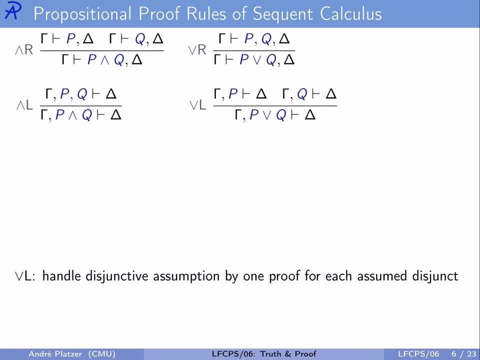 disjunction. We can't know which one it is, but we'd have P or Q among our assumptions. so we know that one of them has got to be true and we covered both the cases. Notice a bit of a duality here: The and left proof rule and the or right proof rule sort of kind of have the same shape. 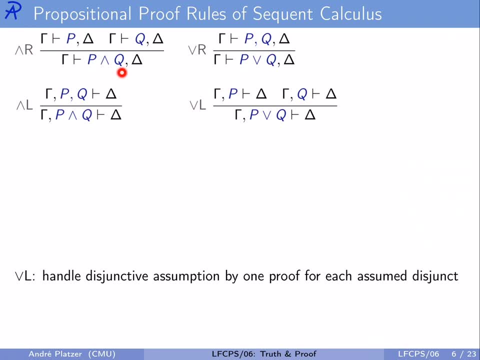 but the or left proof rule and the and right proof rule sort of kind of have the same shape. That's, of course, not a coincidence. you can think about why. Well, that's good, We've got proof rules that handle conjunctions, whether they occur in the left-hand side or 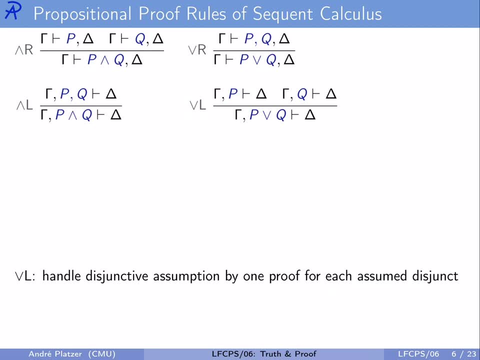 the right-hand side at the top-level position of one of the formulas, and we've got proof- rules that handle the disjunctions, whether they occur in the left-hand side or the right-hand side at the top-level of a sequent. Now you might run into a little bit of a problem. You might run into a little bit of. 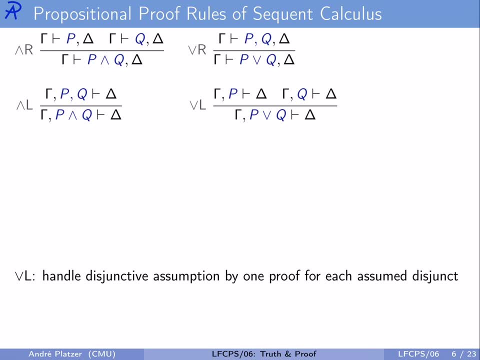 a problem. Other propositional operators are top-level as well and we've done that. in our bouncing ball example even there was an implication operator. But I think- at this point you see our program- that if we find one reasoning principle for each of the propositional 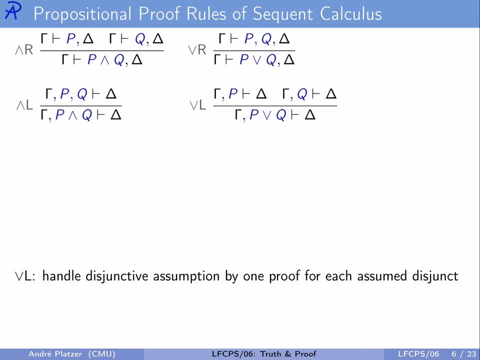 logical operators that we could have both on the left-hand side and on the right-hand side, then we've covered all the ways of possibly reasoning about them. Well, let's go right ahead and worry about how do we prove an implication, The implication. 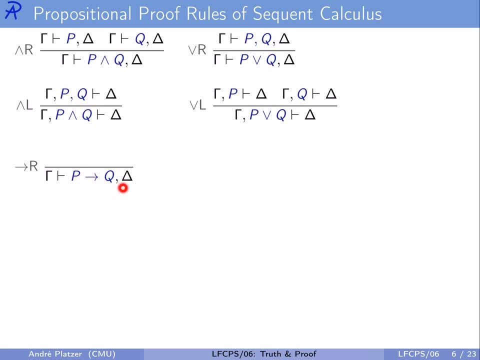 could occur on the right-hand side of the sequent, so somewhere in the succident part, For example, P implies Q or maybe some other alternative which, of course, implicitly is read like: so How do you go about proving an implication that P implies Q? Well, you, 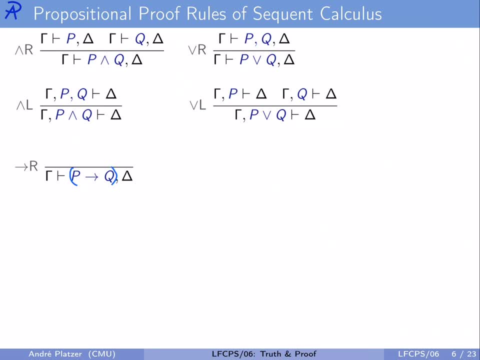 know. if you want to establish that P implies Q, you would assume P go off on the journey to prove Q. That's easy to cover in sequent calculus by saying that from the extra assumption P, together with the old assumptions gamma that we already had, we're now trying to prove. 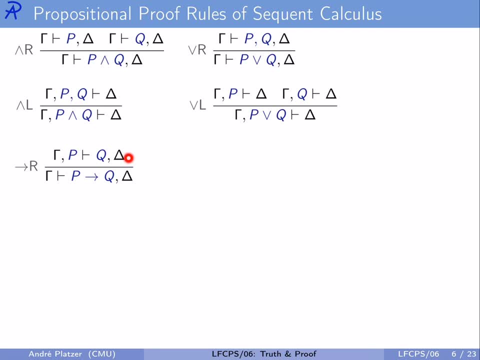 Q from that Well or maybe one of the other things. Seemingly it might look like P implies Q. What does it look like? We're assuming P also here for proving the deltas, which would be kind of awkward. but if you think about it logically, we're not really doing that Because 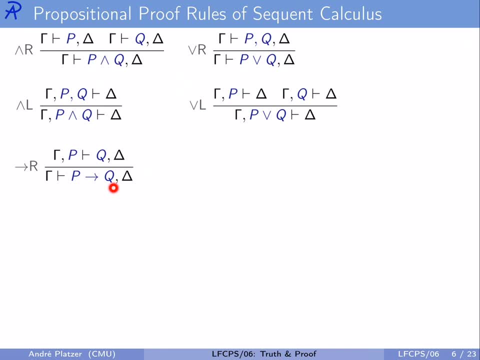 we're merely trying to establish that P implies Q or the other deltas are true. If we assume that P is true, then it suffices to convince ourselves that Q is true or one of the other deltas is true. So if you ever end up in a situation where P is false, then you have already shown that. 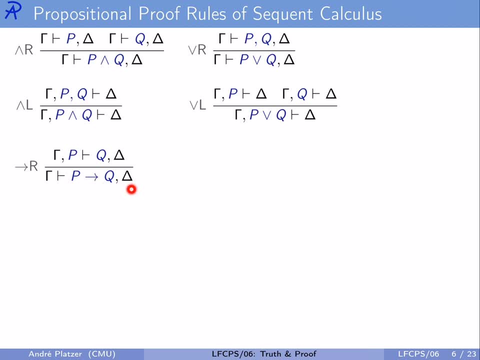 P implies Q or instead, delta works out because you have already shown that P implies Q works out because you have already shown that P is false. This case is actually okay to assume the P here. In other words, the implies right proof rule proves an implication by assuming. 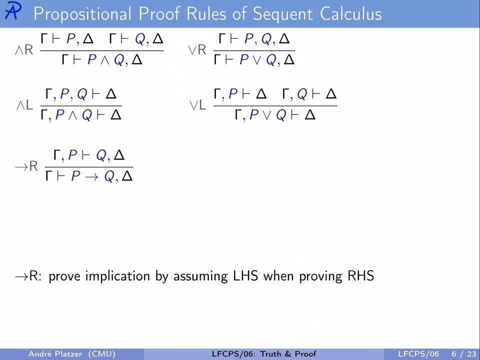 the left-hand side and going on to prove Q. The right-hand side is the one that is going to prove the deltas. The right-hand side is the one that is going to prove the deltas. The right-hand side is the one that is going to prove the deltas. Everything we need to. 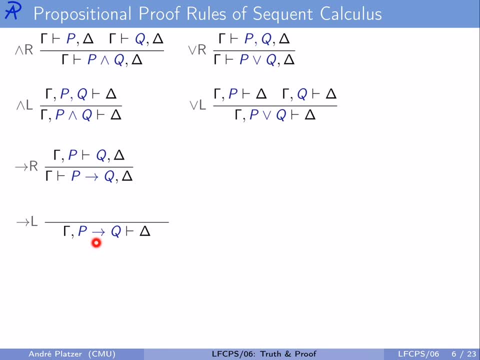 do is assume an implication. If we have P implies Q among our assumptions, how do we proceed with the proof of that? Well, if you have among your assumptions the statement that if something is a prime number, then you cannot divide it by four different numbers, 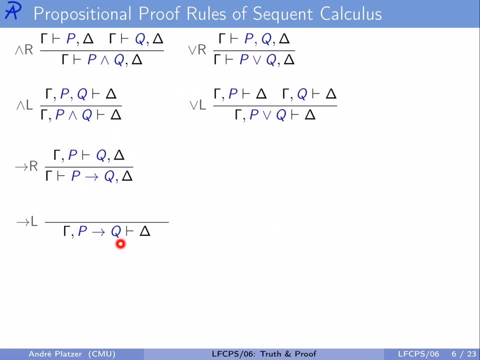 then well, you can continue to work with the assumption that you cannot divide it by four different numbers, but I guess you first go ahead and prove that something actually is a prime number, because otherwise it isn't true. The number 60 you can divide by many. 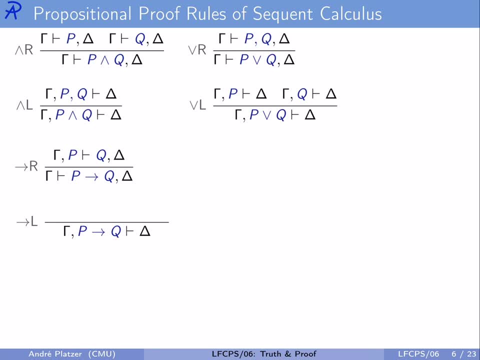 different numbers, but it also isn't a prime number. So how do we make use of an implication among our assumptions? We make use of it by first proving that what it assumes is actually true, Then going on to assume the right-hand side of it instead. Sure thing, because if we know, 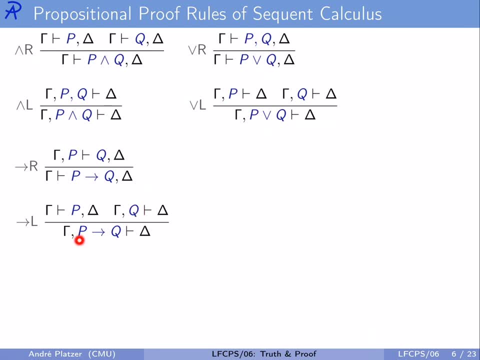 P. well then, we can assume Q from that one, because we already did assume P implies Q among our assumptions here. Now again, I invite you to first worry about the case when the other alternative's delta is the empty set of formulas. but it also works out if you. 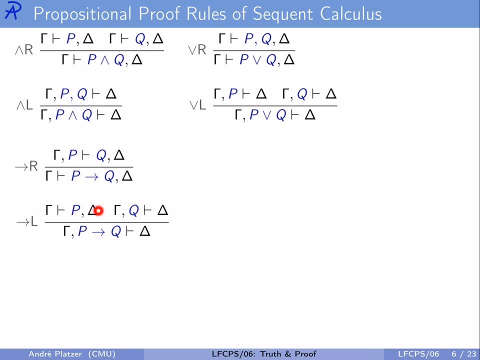 have other alternatives, Because if you succeed with the proof of delta, then you can prove that something actually is a prime number. If you succeed with the proof of delta, then you can prove that something actually is a prime number. So if you succeed with the 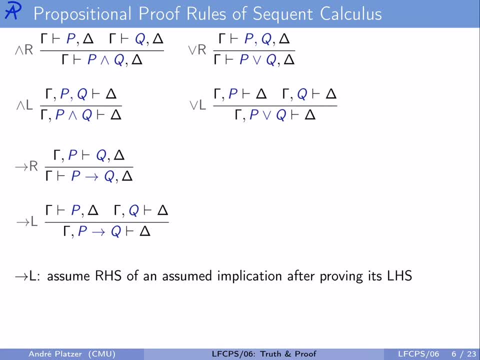 proof of delta here instead and the delta here instead, then of course you can establish that. In other words, the implies-left-proof rule assumes the right-hand side of the assumed implication. P implies Q, but only after it already succeeded with proving the left-hand. 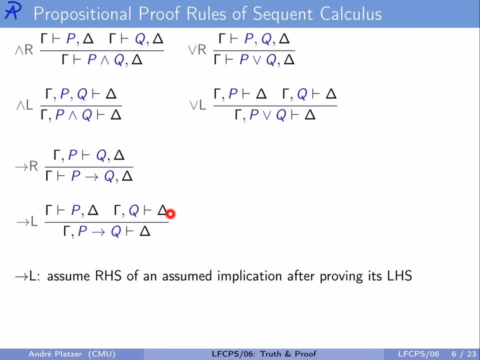 side of it, while keeping the other alternatives open. Now, how do you prove a, not Proving that not P is true or some other things? well, We might as well assume that P is true and then proceed with a proof, for example, of: 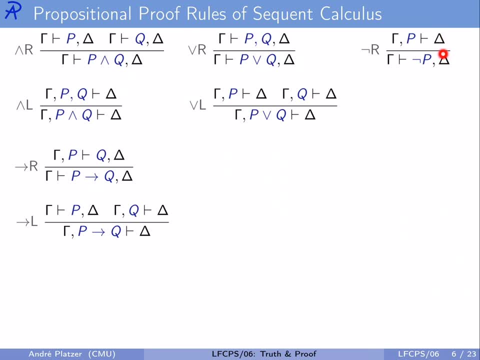 a contradiction. If there are no alternatives- delta, then this is the disjunction over the empty set of formulas, which is just false, just like the conjunction over the empty set of assumptions would be true. Proving that not P is true from some assumptions is the. 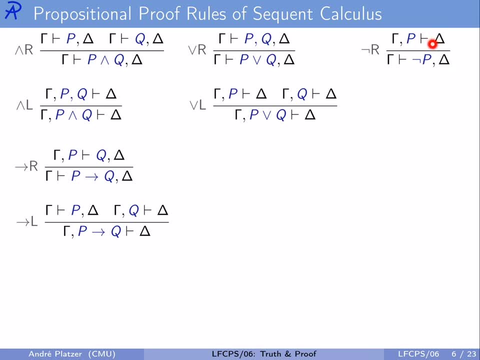 same as well. let's assume P and prove a contradiction from that, then I guess we prove not P, classic logic. But the same thing also works out if we keep other alternatives around. Because again, if we have succeeded in the proof of delta already, then also down here. 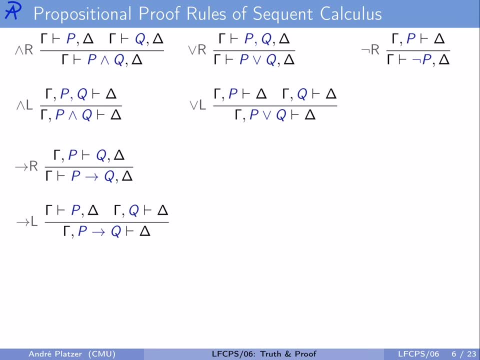 we've succeeded in the proof of delta. never mind that not P is one of these, So you can also understand the not right proof rule just by reminding yourself about the meaning of the sequent, which is: the conjunction of the left-hand side implies the disjunction. 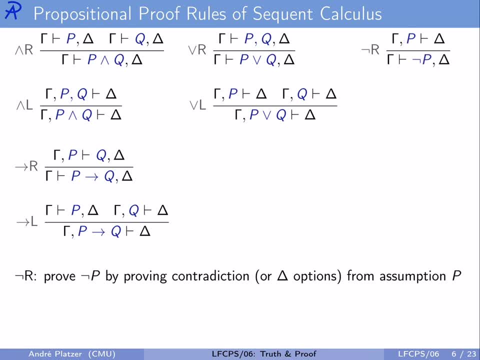 of everything on the right-hand side. and then you see this duality. So you prove a, not P, by proving a contradiction. nor do you have a delta option from the assumption P. If you assume a negation, not P, among your assumptions, then you can also prove a not. 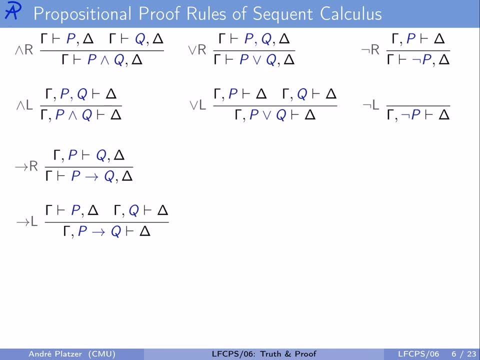 P. Well then you can also just prove P, which is the opposite of, not P- from the assumptions, Because if you have a proof of P from your assumptions, then of course you also have a proof of contradiction from the extra assumption- not P. The same thing also works out still. 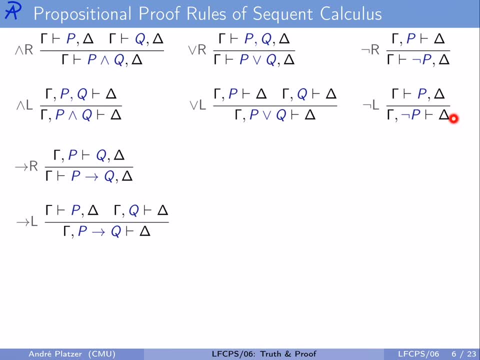 if you have other alternatives, delta. instead of proving a contradiction from that, Again, I invite you to look at the implicitly-alternative delta. It's the implicitly-implicative, conjunctive and disjunctive meaning of sequents. in order, 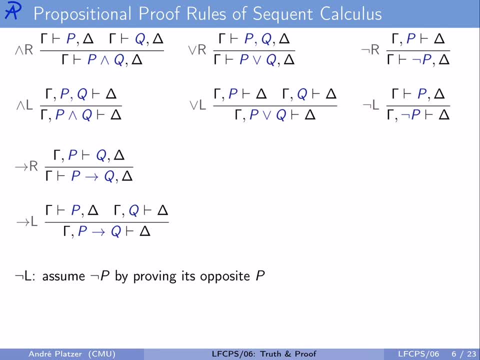 to understand these two proof rules. Overall, we're assuming a negation by proving its opposite form instead. Now all of these proof rules. they handle logical connectives on the left-hand side and on the right-hand side of a sequent. Oops, we forgot about, by implication, P, if 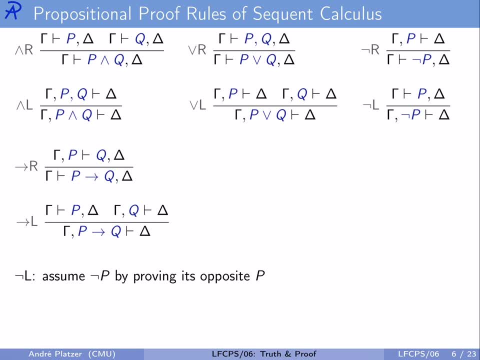 and only if Q, But P if and only if Q, P if and only if Q is also the same as P implies Q and Q implies P. I guess it's already covered, But even if these now all structured our thinking, all of these proof, rules, applications from: 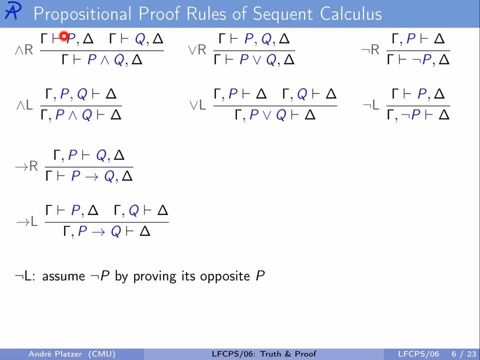 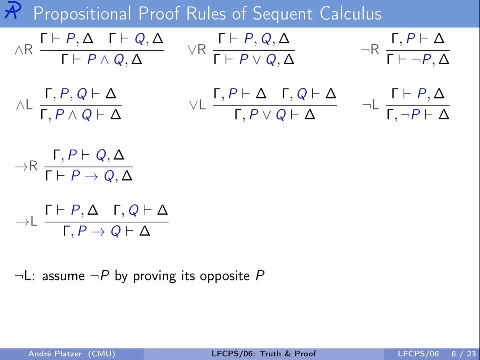 it's really valid, so true in all states. When is that syntactically obvious? It's syntactically obvious that a sequent is valid if, among our assumptions, if along our assumptions, it is proven that the��feel is capable of proving a sequent. 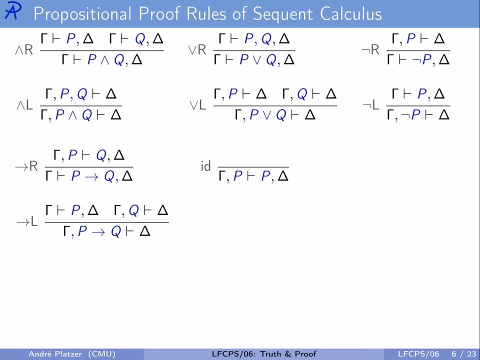 we find what we're trying to prove. Here's the proof rule for the job. If among our assumptions and the antecedent we find a formula P that we also find among the things we're trying to prove, then certainly does P follow from the assumption P, never mind what Gamma did. 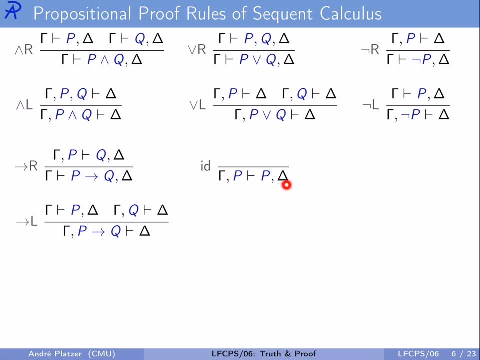 and never mind whatever alternatives delta are there. In fact, there's nothing left to prove by this identity proof rule In order to make sure, in an actual proof, that people realize we didn't just stop writing, but we're really done with the proof we often mark. 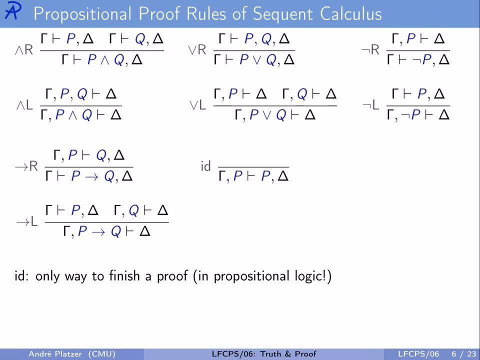 them by a little asterisk. In the use of this proof rule, we would write up here that we're done with the proof which we mark like. so Another proof rule is the logical cut proof rule invented by Gerhard Gensson, which instead: 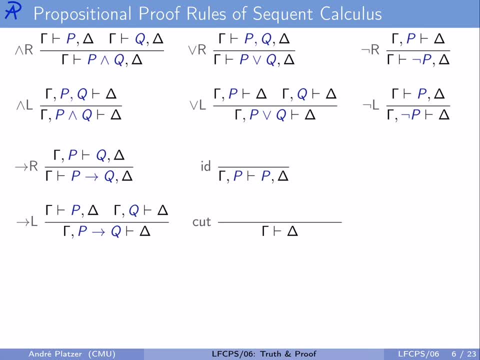 of like all the others, basically make a case distinction on what logical formula we've got proves that delta follows from Gamma in a different way, by first proving that a formula C follows from the assumptions Gamma and then assuming that C holds Again first. 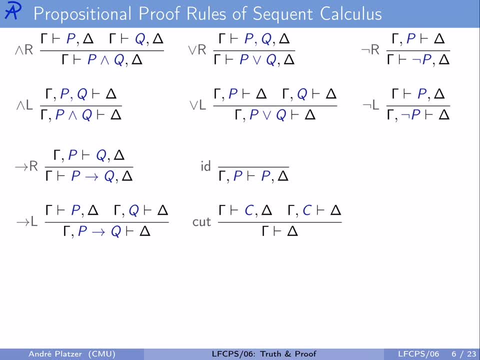 I invite you to ignore this delta alternative here. and then the cut proof rule says that C follows from Gamma. If we assume C in addition to the assumptions we already have, then the original delta can be proved. That's actually like a lemma: We first prove the lemma C and then we assume. 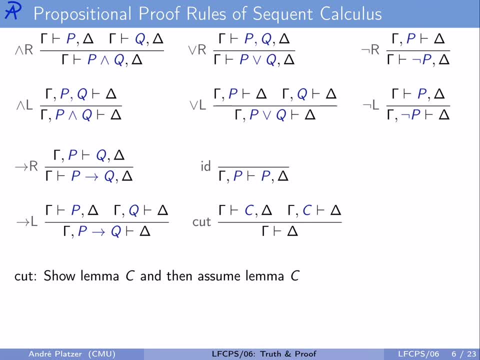 within the rest of the proof, and that makes all the sense in the world. Now let's worry about what happens if there's this delta here. Well, if we find a proof of this sequent, we have not really succeeded. We've succeeded in showing that C follows from the assumptions Gamma, because we could 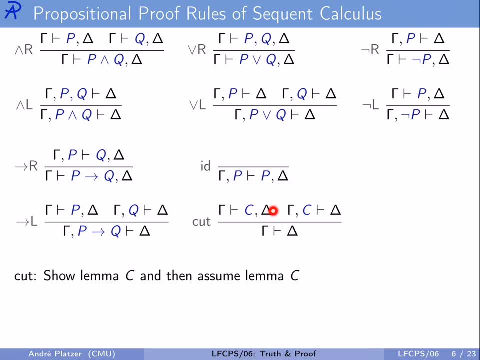 have come up establishing that delta is actually true or one of the alternatives, and then we don't know that C is really true as well. But that's fine, because if we have established delta from these assumptions, then well, we've established delta from these assumptions. 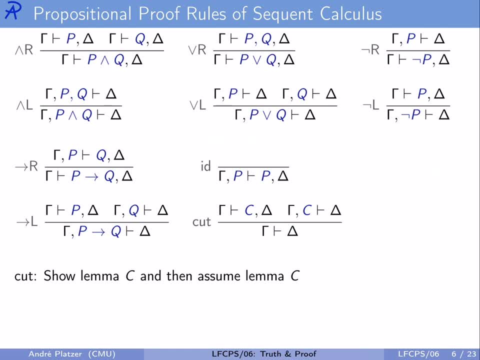 and then we're done with this proof part as well. Now we're essentially done with all the propositional connections, But let me just be very explicit about two that we won't really use, but you should know about them. The true formula, the formula that's just syntactically true. so it also. 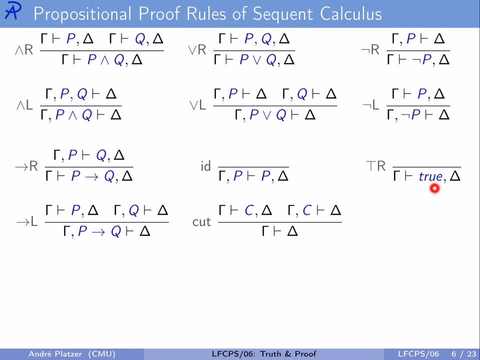 semantically is always true, no matter what state. How do we prove that? How do we prove that true is true from some assumptions? Well, we're already done with the proof, because the true formula is always true, no matter what state we're in. 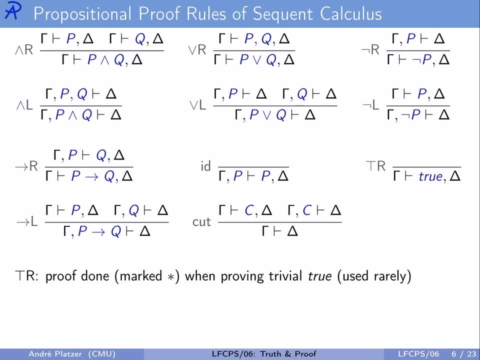 So this has its own proof. What do you do if you find a true formula in the assumptions on the left-hand side? Well, you can't make use of the assumption that the formula true is true, because it's not a very helpful formula, because you didn't put any knowledge into establishing that the 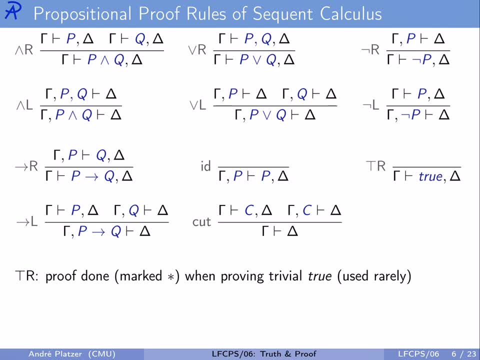 formula true is true. In other words, there isn't much you can do with the formula true, except that it's a proof rule that occurs among your assumptions. you can basically ignore it. We'll see later on how we do that in a proof rule directly. 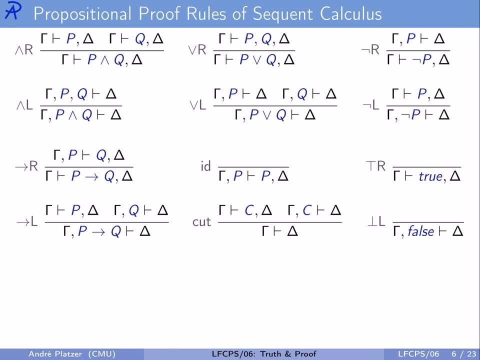 If we have the formula false among our assumptions on the left-hand side, then how do we prove that delta is true from the assumptions of the gamma and then false? Well, again, we're done, because if, among all the other things that are false, we have the delta, then that's. 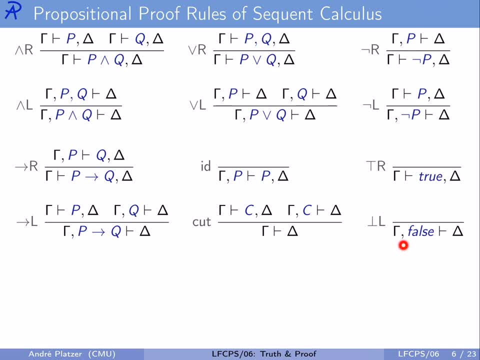 false. So that's the proof rule. Okay, so that's the proof rule, Okay. Okay, we're assuming. we're also assuming false. well then, anything follows from that, because the formula false by definition is never true in any of the states. So it's one of the 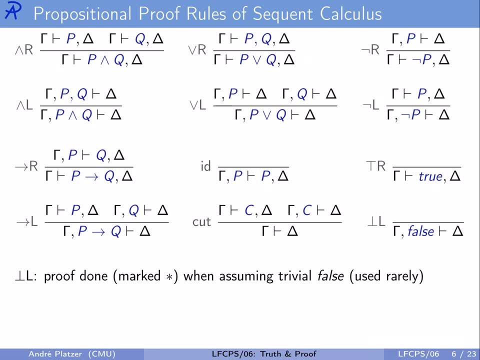 by definition, false assumptions. so we don't have proof. How do we go about proving false on the right-hand side? so that's the false-right proof rule. No, no, no, no, hold on a moment. We're never actually supposed to prove that false is true, because the entire point is: 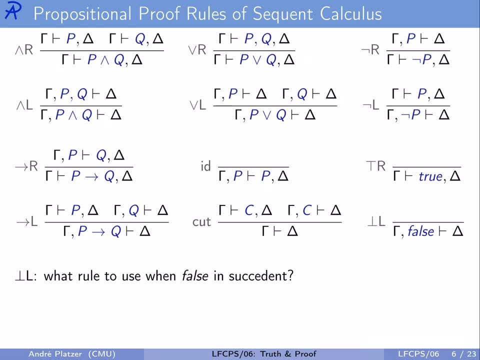 that the formula false is always false in all the states. So there is no way of proving false except in the cases where false is already among our assumptions. So, for example, the identity proof rule. It would enable us to prove false, but only if false is already among our assumptions. 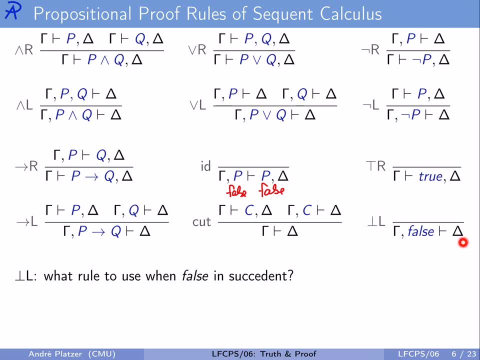 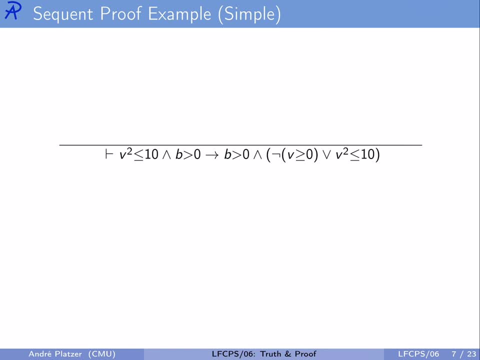 And, of course, if we have false among our assumptions, then anything follows from that. even false itself does. Let's put these proof rules to some good use. So here's a logical formula that absolutely deserves a proof. Hold on a minute. It only deserves a proof. 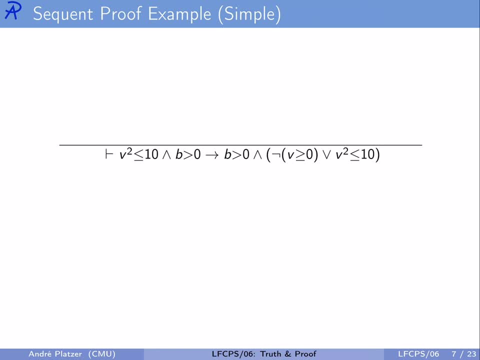 if it's really valid, so it's true in all states. That's what sound sequent calculus proof rules will be able to tell How do we go about proving it First, we turn it into a sequent, so we add the sequent. 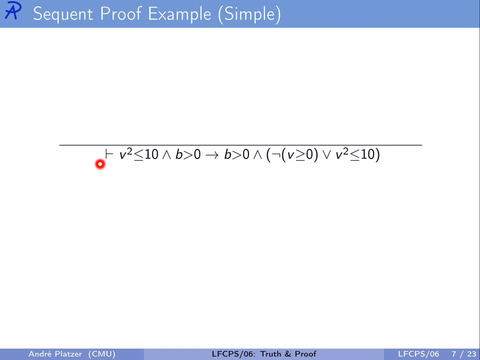 turnstile in front of it and prove it from no assumptions. Notice, we've got no assumptions when we're trying to prove this. What can we do with it? Well, the logical formula tells us what we need to do to prove it, because its top-level operator is the implication. 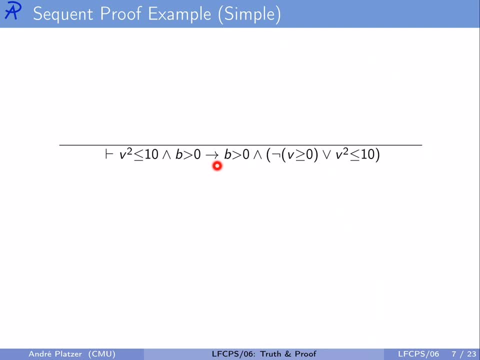 operator and we of course prove implications that occur on the right-hand side by using the implies right proof rule, which proceeds by assuming the left-hand side to prove the right-hand side. We've reduced the question whether this sequent has a proof to the question. 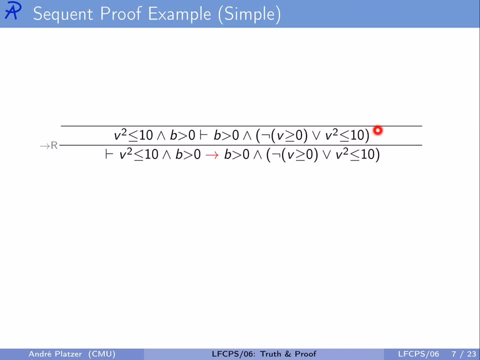 whether that simpler sequent has a proof. Why is that simpler? Okay, Well, because it has one less logical operator, and if we keep on deleting logical operators, at some point it's going to be really easy by the identity proof rule Now. 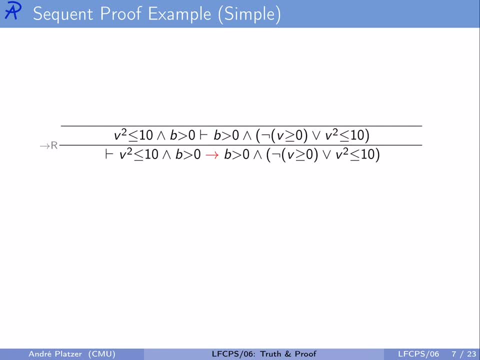 how do we prove this sequent now? Well, it has a conjunction on the right-hand side. How do we prove a conjunction on the right-hand side? By the AND right proof rule, which? what does it do? again, It proves each of the conjunctions separately. We will have to ask: 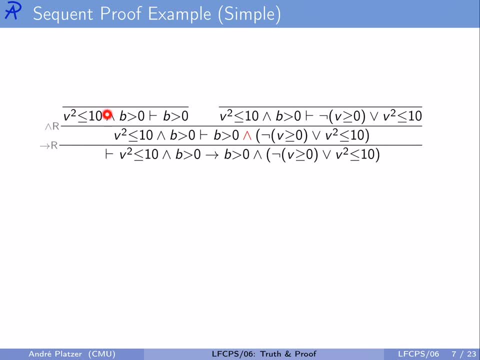 ourselves. does B greater than zero follow from the assumptions we used to have, and does the other formula follow from the assumptions we have? What do we do here? Now? we've got two sequences of questions. On the left, one we really ran out of clever things to do on the right-hand. 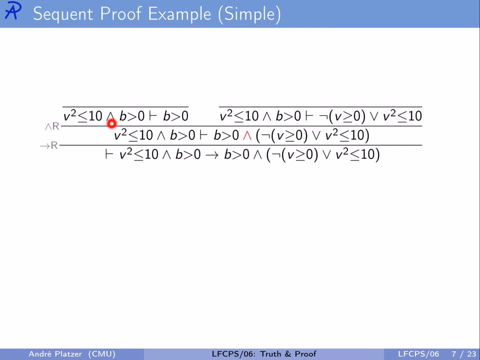 side. We look into our assumptions and find that our assumptions still have propositional structure. We're assuming a conjunction here. How do we proceed about proving a sequent in which we are assuming a conjunction By the AND left proof rule, because the AND is on the left-hand side, The AND left proof. 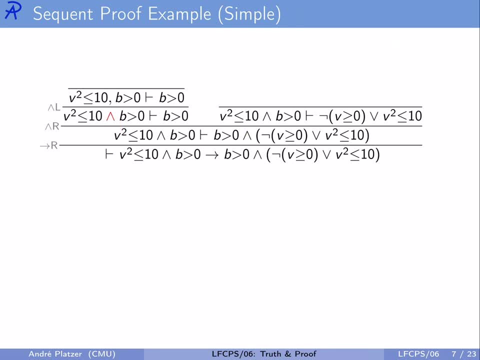 rule, of course, assumes each of the conjunctions separately. We assume this and we assume that. to prove this, What do we do now? We're done because among all of our assumptions do we find what we're trying to prove? That should be really easy by the identity proof rule. 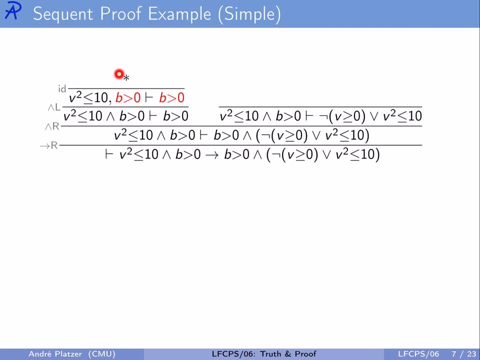 We mark that we're done just to remind ourselves that we didn't get to keep on writing just like we did over here by writing down the asterisk star here From B greater than zero. of course, B greater than zero follows, even if we assume other things. Yeah, so we're. 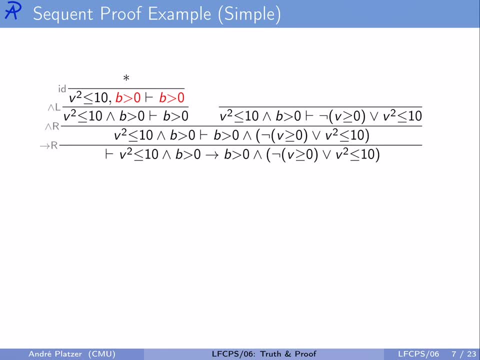 done with the proof Now? we're not done with the proof. We're only done with one of the branches of the proof. Of course, the sequence at the bottom will only have a proof if the entire sub-questions that we're asking here are true. 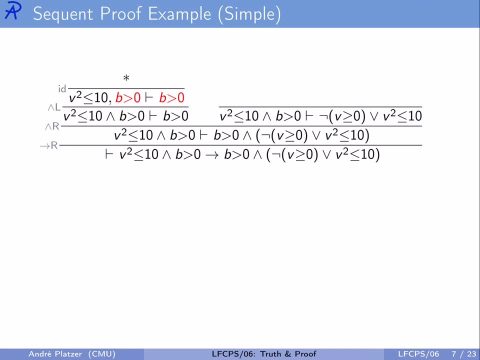 here have proofs. This one now does have a proof, but that one doesn't yet, So I guess we need to worry about this. We have a disjunction on the right-hand side. How do we prove a disjunction on the right-hand side? By the or-right proof rule, which just lists all the 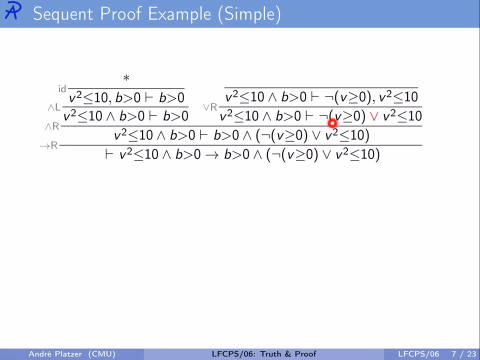 options separately to proving that not v greater or equal 0 or v square less or equal 10 is the same as just proving that this or that follows from our assumptions. Now we could be worrying further about the not operator on the right-hand side, but maybe 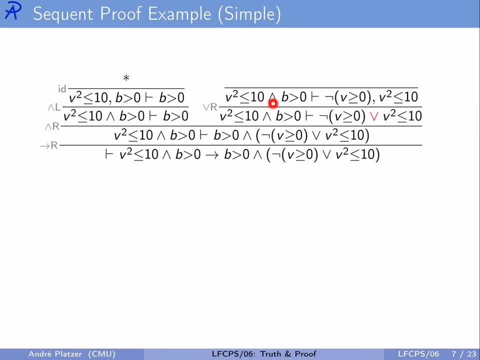 you already see that it's more clever to think about the assumptions that we have here, because our assumption actually seems like it's including what we're trying to show here. So we can worry about how do we work off an assumption that is a conjunct. 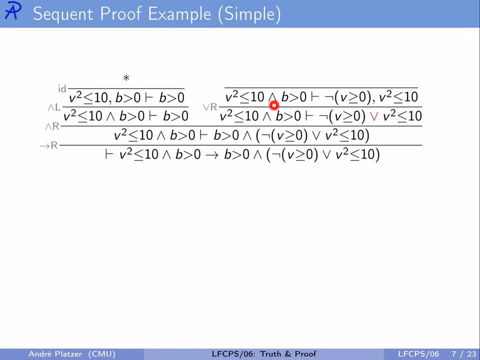 Well, if we have an and on the left-hand side, then we prove that using the and-left proof rule, which assumes the two separately. So we assume the left conjunct and we assume the right conjunct separately. and now it's real easy. Now, among our assumptions, we find: 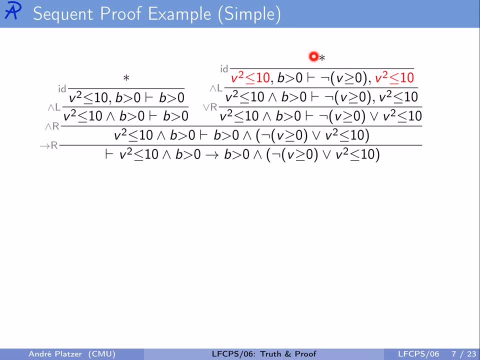 what we're trying to prove. So by the identity proof rule, we're done. Now we need every part of the proof is done. That means because each of the proofs professors- Now the first proof we've used here was a sound proof rule- that if all the 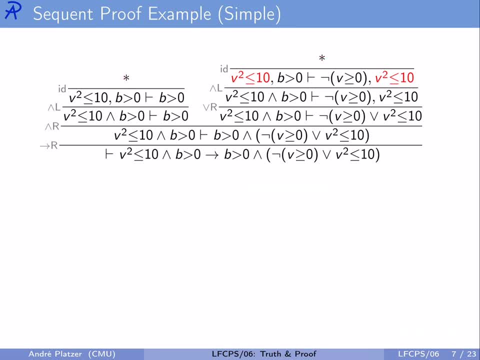 premises of the proof are sound. Actually, there are none. This is just a mark that we're saying we don't have any more premises to we worried about. The empty set of premises is valid in every state, because they don't even impose any conditions, Because they are. 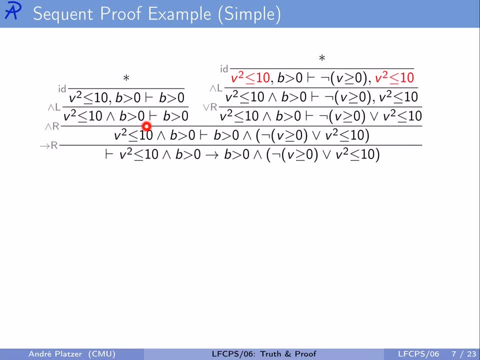 because this was a sound proof rule, the conclusion is valid. So it's conclusion because it was a sound proof rule is valid. It's conclusion because it was a sound proof rule. so the conclusion is valid and it's conclusion because it was a sound proof rule is valid and the conclusion is valid, which means that, actually, when this consumers performed a little more work ‑‑ that this is true and that it's a result. there is an absolute majority ofứngfor being true or false, because it's not valid In one or two solutions. 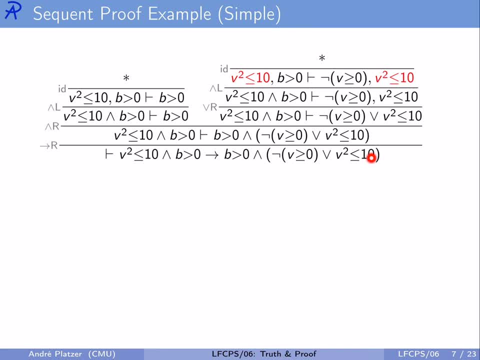 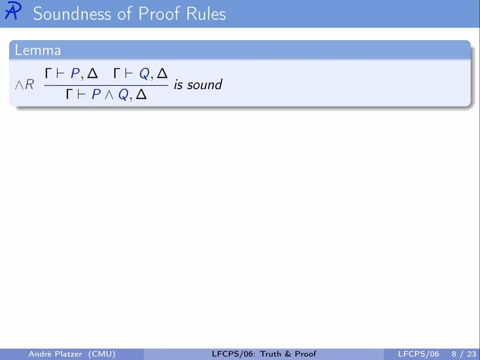 conclusion is valid because they are da-da-da-da-da. The original question is valid. if all of the proof rules were sound, which is the next thing we should be worrying about, We could have written down proof rules that were just nonsense. What does it mean again for a proof? 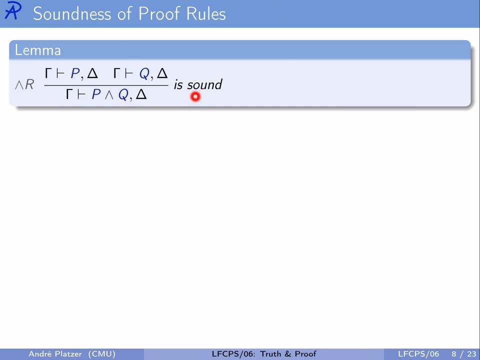 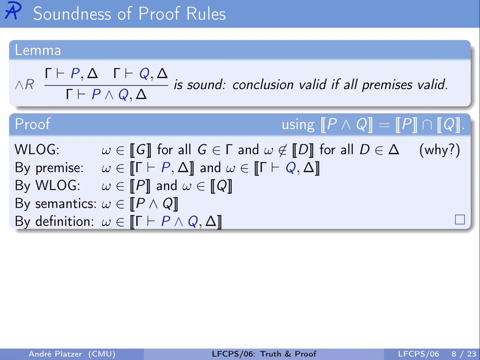 rule, for example the AND write proof rule, to be sound. It means that if all the premises are valid, then so is the conclusion. Let's convince ourselves about that, that the conclusion is valid whenever all the premises are valid. We do that from the semantics If we want. 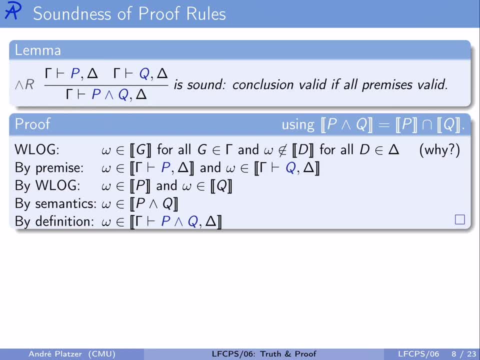 to convince ourselves that this sequence is valid. we might as well assume that all the formulas in gamma are true in a sequence, The state omega that we are considering, because if in that state one of the assumptions in gamma is not true, then the entire sequence is already true because it says: if all kinds 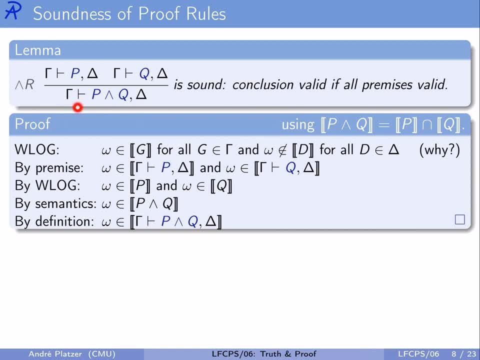 of things are true that aren't true, well then, any arbitrary thing follows. Remember, the meaning is an implication. We might as well also assume that in this state, none of the formulas on the right-hand side, delta, is true, Because, again, if one of them would, 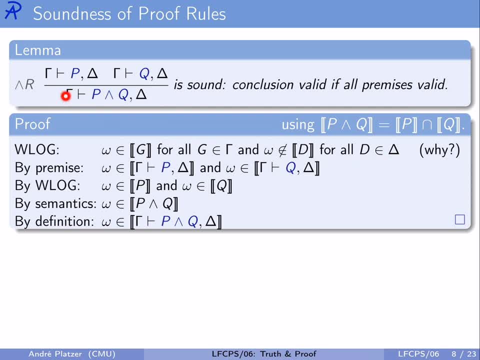 already be true, then it's not true. Our overall implication meaning, which has a disjunctive meaning of the comma on the right-hand side, would already be true. It's really only interesting if we are in a state where all the gamma assumptions are true and none of the delta assumptions are true. Now, 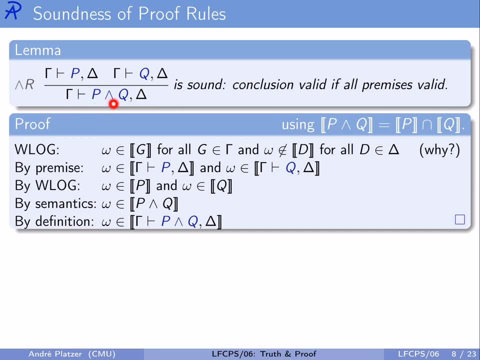 we really need to establish that P and Q is true in the state omega. That we cannot possibly show without looking at the only thing we've got, the premises By premise. we know, in particular in this state omega, that the state omega is true. That's the only thing we've. 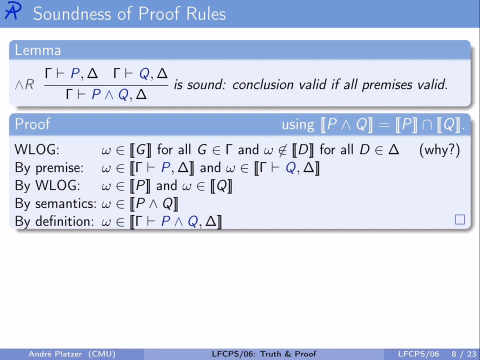 got the premises. So by premise, we know, in particular in this state omega, that the state that we care about, that the sequent is true, or rather the logical formula that is corresponding to this, The one that says conjunction of all the left-hand side implies: 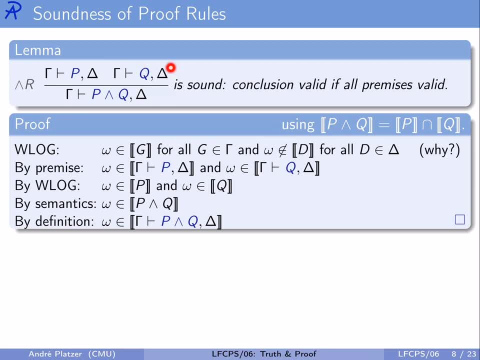 disjunction of everything on the right-hand side Likewise. well, this is valid, So it's also true in the particular state omega. Now, by what we assume, we've had loss of generality here. all the gammas are true in the state omega. 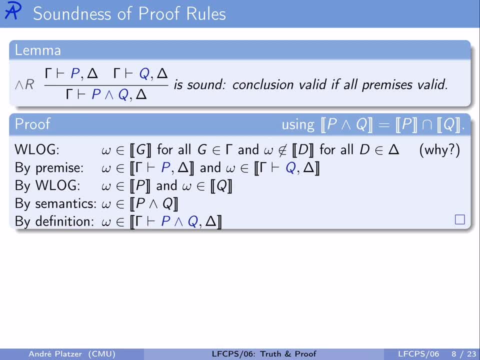 But none of the deltas is So. the sequent can only be true in this state if P is also true in this state. This can only be true in this state if Q is also true in this state. That means by this left premise. do we know that in the particular state, omega does P? 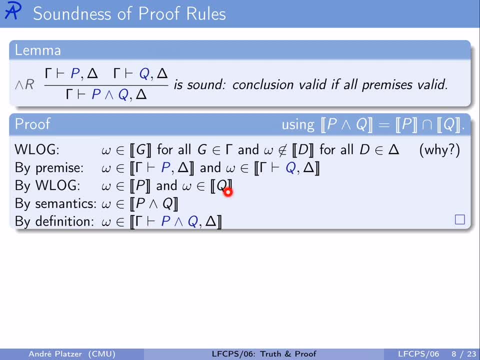 have to be true By the right sequent. do we know that Q has to be true? Well, and then we of course know that their conjunction, P and Q, is true, because that's the meaning of conjunction. Remember the set of all states where P and Q is true is. 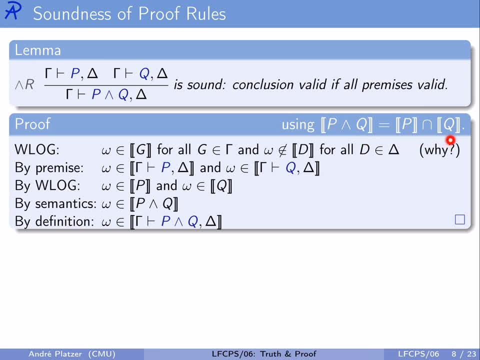 just the intersection of the set of all states where P is true with the set of all states where Q is true. So both P and Q are true in the state omega, so is the conjunction Well, and that of course means that the sequent that we're trying to establish is: 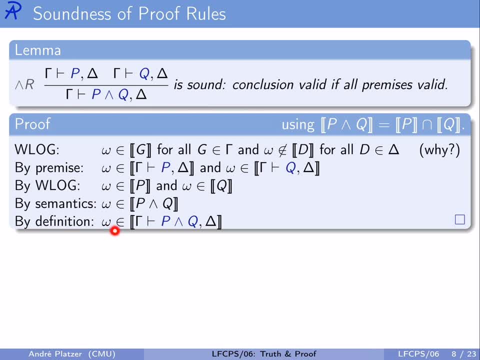 true in the state omega. And hey, that state of omega was completely arbitrary in our argument, so of course it works for every state omega. so the sequent is valid In similar ways. the following is true: Of course it doesn't suffice to just convince us at the end. right Proof rule was a sound. 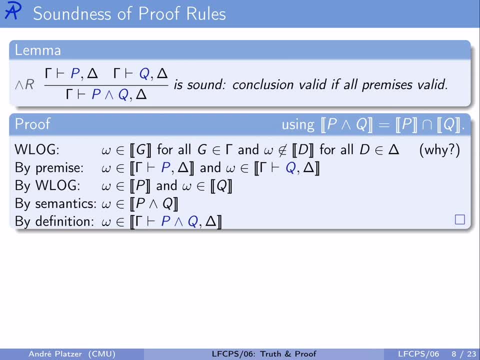 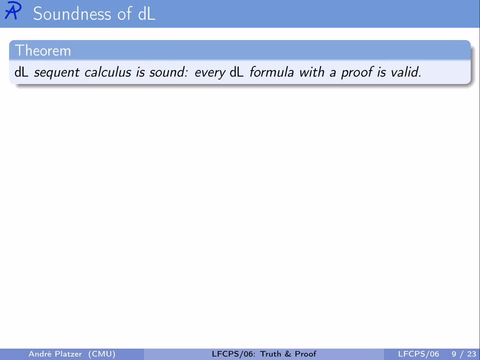 one, but all of the proof rules we ever adopt have to be sound. Then we're able to prove the theorem of soundness of sequent calculus that every differential amygdala logic formula with a proof is actually valid. This, of course, is very important. Imagine you're going off. 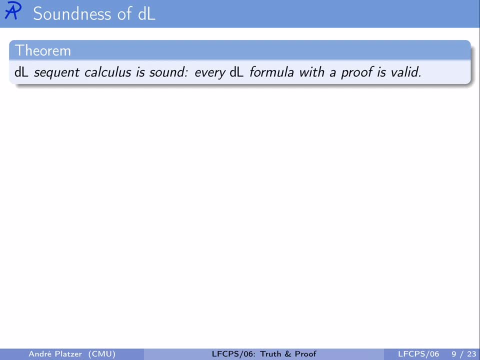 on a journey to find a proof for your favorite subphysical system, and you do that. you write down something that claims to be a proof. You say proof because you use all kinds of proof rules and you find out that, regardless, the conclusion at the end isn't really valid. That would be very annoying and very awkward. 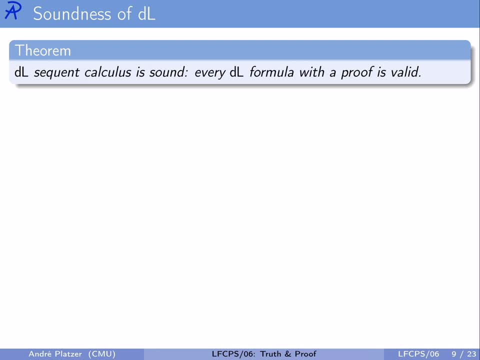 because you would have just proved something counterfactual and would have established the safety of a system, signed off on it, without it actually being safe. That's very bad, But in logic we can convince ourselves that indeed, every time we say there is a. 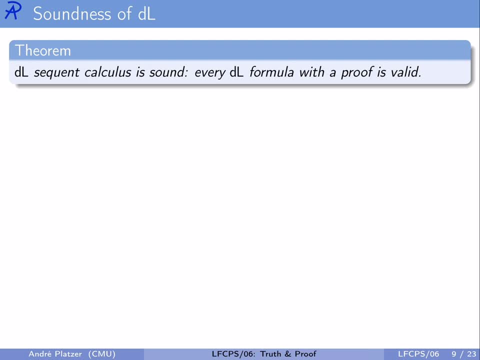 proof, the conclusion of it is really valid. But how do we prove this soundness theorem? Well, every differential amygdala logic formula with a proof is supposed to be valid. but how do we prove differential amygdala logic formulas in sequent calculus? Well, by first converting them into a sequent and then having 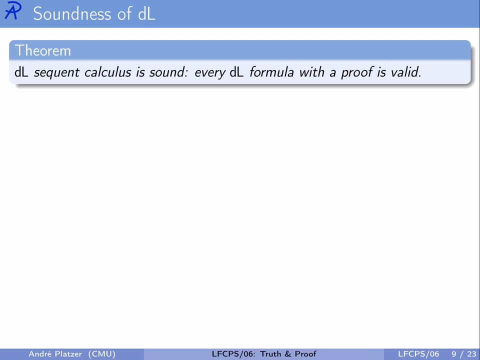 all kinds of assumptions in the left and all kinds of formulas in the set-size of the right. In other words, what I'm trying to say is that the way to prove amygdala logic formula, differential dynamic logic formula, is by way of working with its sequent version, and then 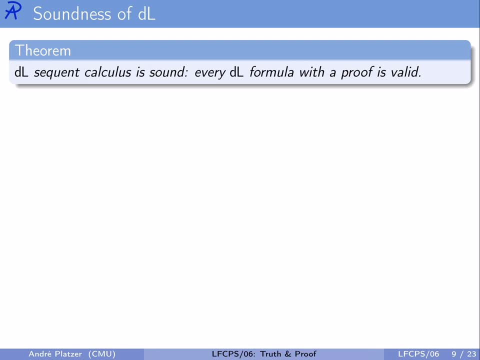 they will internally again work with sequent versions. In other words, what we need to do is to prove in a slightly stronger form of soundness, namely that not just every differential dynamic logic formula with a proof is valid, but every differential dynamic logic sequent. 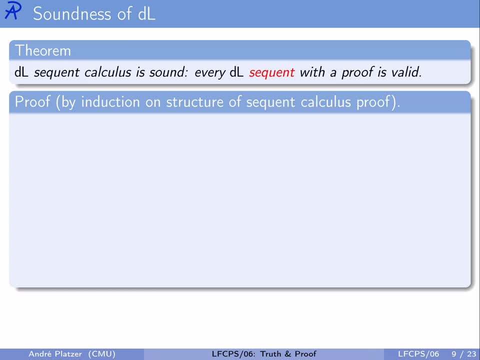 with a proof is valid. If there's a proof of a sequent, then the sequent represents a valid formula, which we do prove. that's the beauty of logic: by induction on the structure that the sequent calculus proof has, We know the shape of the sequent calculus proof: It's: 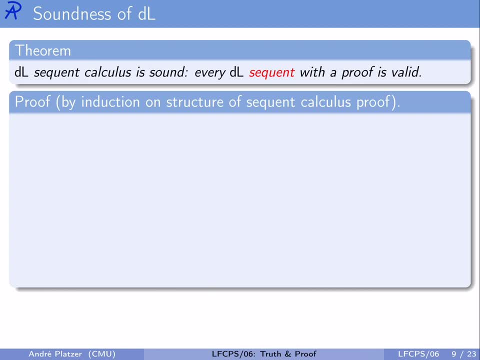 going to be some set of proof rules applied in a bunch of places. We know all the proof rules, We wrote them down, Admittedly only the ones for propositional logic so far. but we should first understand soundness of the propositional case. 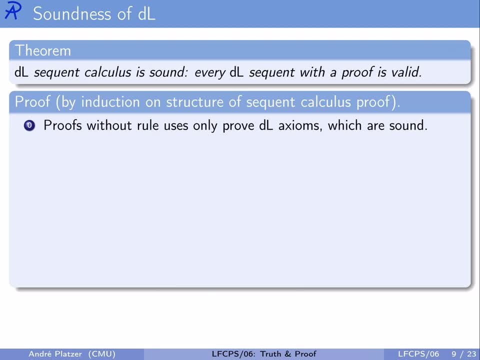 Well, we could do that. We could have started from nothingness. We could have started with the simple most proofs, the ones that don't use any proof, rules, which are just the ones that are axioms, because differential dynamic logic axioms are the only things we can prove without using any. 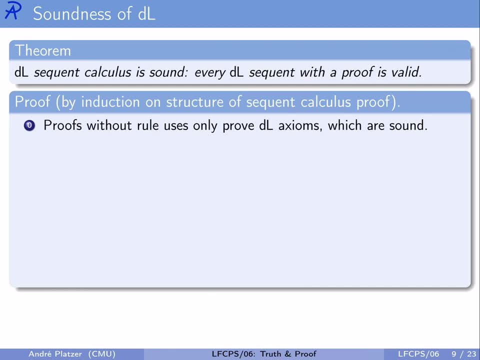 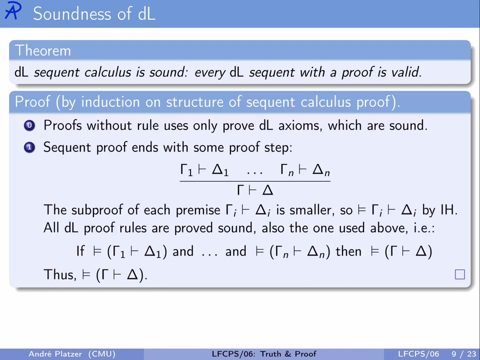 proof rules. We've seen last time that each of the differential dynamic logic axioms is sound, which means all their instances are valid formulas. Well, valid formulas are valid formulas even if you write a sequent calculus symbol in front of it. That's easy. It could have been a proof that consists of having applied a sequent calculus. 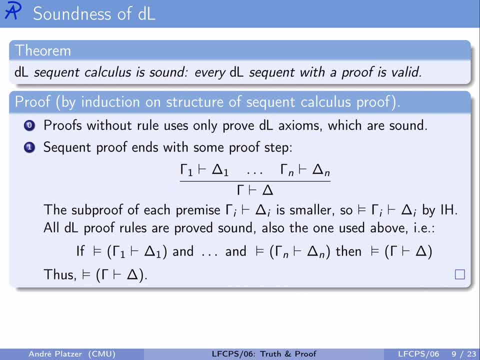 proof rule. Here's one proof rule step. There could have been more here, could have been more here, but at least this one proof is smaller than the entire proof. and this one proof is smaller than the entire proof because both the proof on the left and the proof on 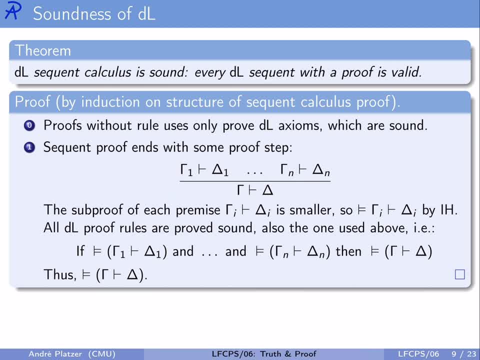 the right and everything in between are missing at least one proof rule application Now by induction hypothesis. this has a smaller sub-proof, so if it has a proof by induction hypothesis, this is a valid sequent, and so is that Now all the proof rules? 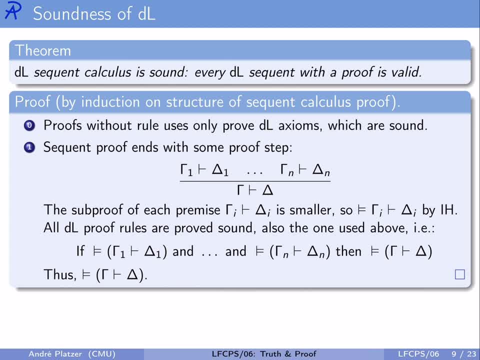 we could have been using in sequent calculus for differential dynamic logic are individually proved sound. We saw one proof for the AND left proof rule right now, but of course we also have done proofs for all the other sequent calculus proof rules. That means soundness, remember, if all the premises are valid which we just established. 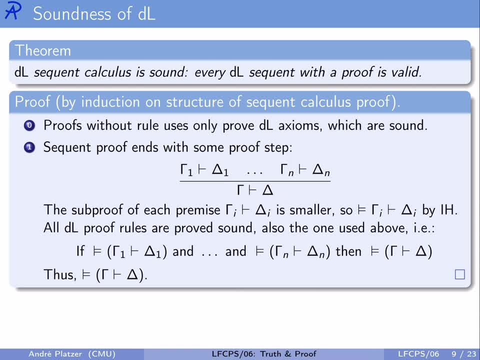 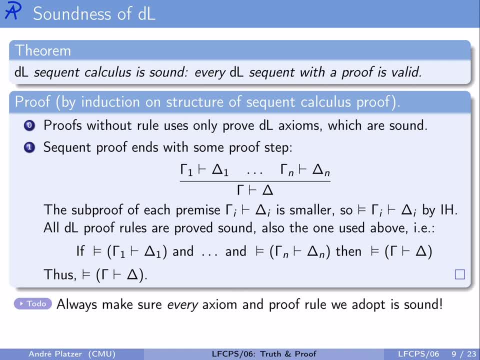 Now, in order to prove soundness and unity, of course we have to make sure that absolutely every axiom and proof rule that we adopt we first need to prove sound, But then we've got a completely compositional soundness argument for every proof, no matter how big we make. 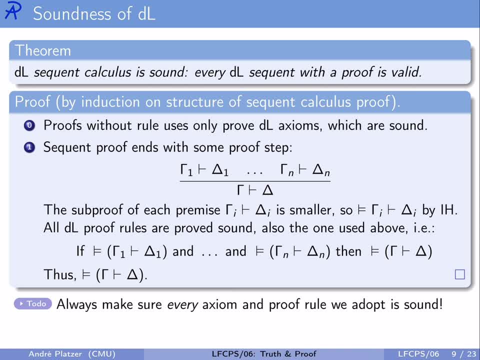 it could be a terabyte of a proof. Each and every one of the axioms was a sound one and we have a finite list of axioms. Last time we saw on the order of 10 or so. Each and every one of the proof rules has a sound one and we have a finite list of axioms. Last, 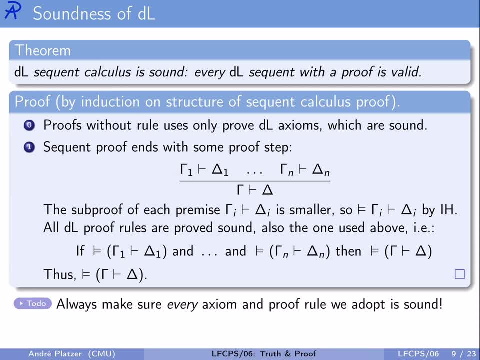 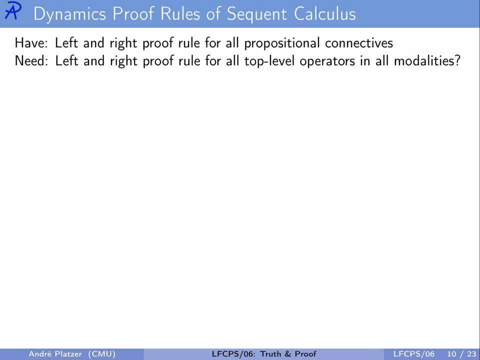 rules- well, now we saw maybe 20 or so also is sound. That means everything is preserving validity. If the premises are valid, then so is the conclusion, which is what we're interested in. All right. so what have we got? We've got proof: rules for ands and ors. 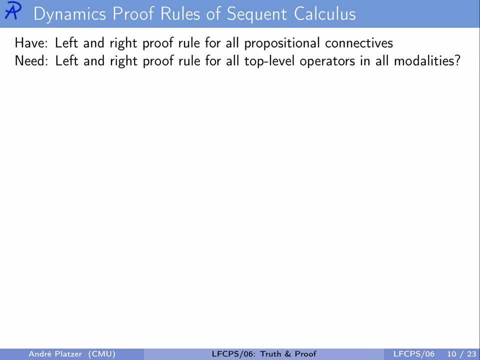 and all the propositional connectives, but we don't have proof rules for any other operators. In particular, we don't have proof rules for modalities. Well, so I guess we've got left and right proof rules for propositional connectives, so we should be doing left and 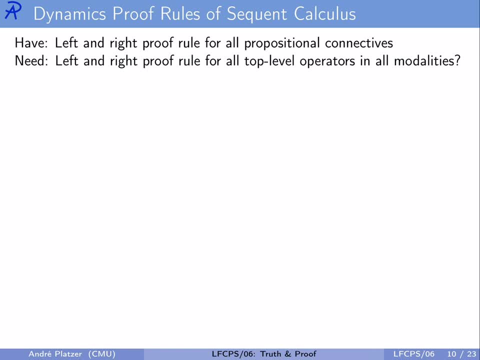 right proof rules for all the other top-level operators, in particular all the modalities, in particular all the top-level operators within the modalities. So I guess let's march right on. We need to develop a proof rule for proving that all behavior of 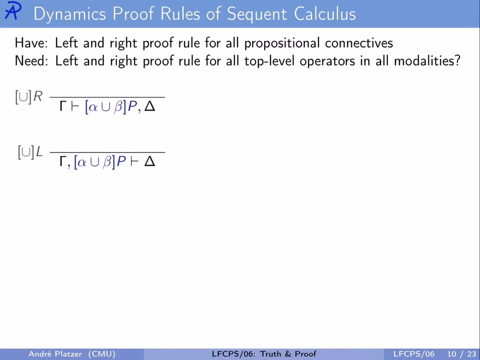 a system that has a choice between alpha and beta is safe. How do we do that? Well, if you want to show that, I guess we need to show that all the alpha behavior is safe and, independently, all the beta behavior is safe. That makes sense to us. What do we do? 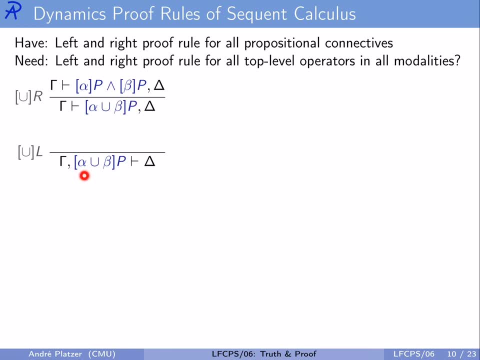 if we find the same formula in our assumptions, The formula that says all behavior of alpha choice, beta are safe. Well, we need a proof rule for the box choice operator occurring on the other side. What do we do? Well, we also say that we work off this assumption. 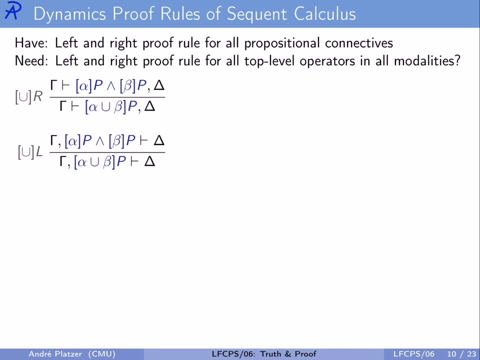 by instead assuming that all the alpha runs are safe and separately assuming that all the beta runs are safe. Of course they're saying the same thing. Is there something That's incredibly boring? because we already know all of this from just the differential dynamic logic axiom of non-deterministic choice that says: 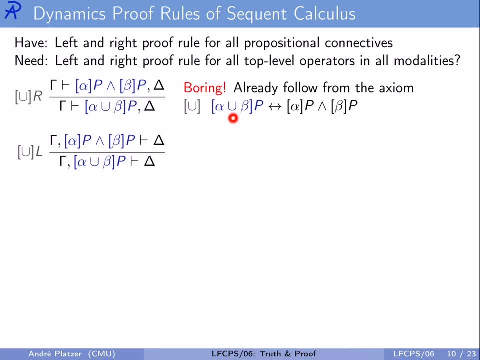 never mind what context. all runs of alpha choice beta are safe if, and only if, all the alpha runs are safe and independently all the beta runs are safe. The two formulas are equivalent, Whether they occur here on the right-hand side of the sequent, or whether 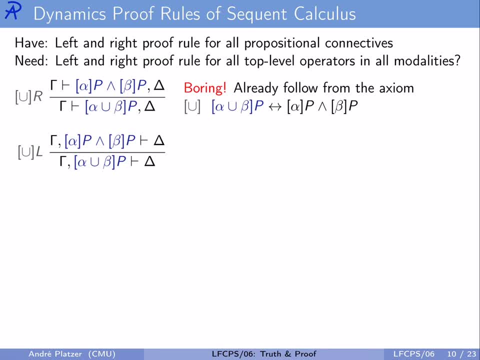 they occur on the left-hand side of the sequent or, in fact, whether they occur anywhere at all. speaking of anywhere at all. these two proof rules, we could be adopting them, but then we cannot use them in another logical context, such as, let's say, in a logical 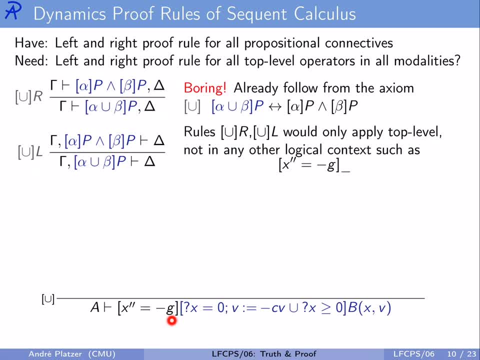 context. This is the one we find after a differential equation. Just look at this: After this differential equation for the bouncing ball, we really wanted to split this non-deterministic choice because it makes our reasoning easier. But this proof rule will not apply here. It's. 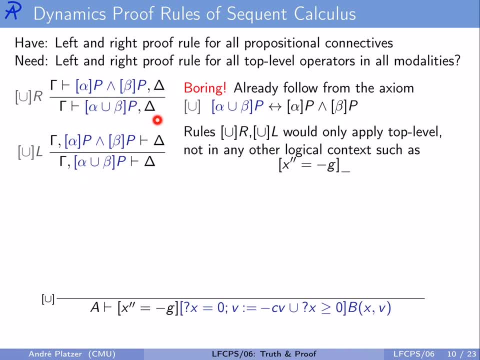 not of the form that one of the formulas on the right-hand side- well, there is only one- starts out with a box choice. No, it does not. It's sort of a differential equation, So the other one, of course, can't. 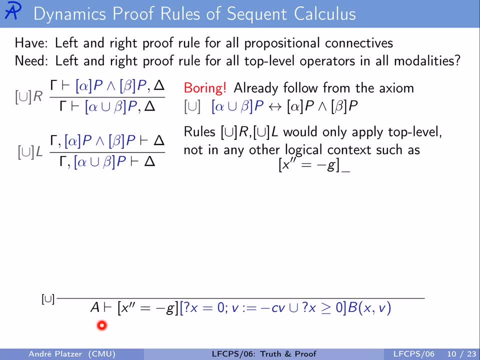 It cannot apply to this either, unless we happen to find this in the assumptions A, which we don't, because these are arithmetic assumptions in this case. In other words, not only would it be very annoying to develop a right and left proof rule for each of the modality operators, 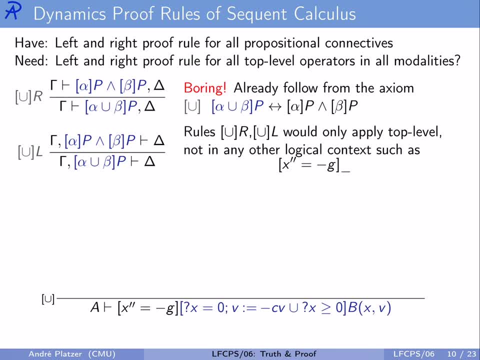 and each of their top-level operators. but also we wouldn't exactly learn a whole lot of new things, because we know all of these things from the differential dynamic logic axioms of dynamics already, and the proof rule would be less powerful. So instead what? 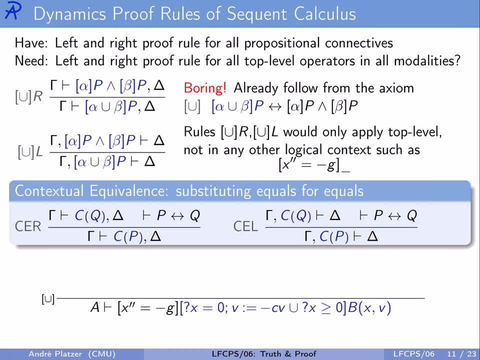 we do. we do this Is we institutionalize the principle of substituting equals for equals. Well, substituting equivalent formulas for equivalent formulas. If in any context, we find the formula P and we know by proof that P and Q are equivalent, for example, like here, then we might as well. 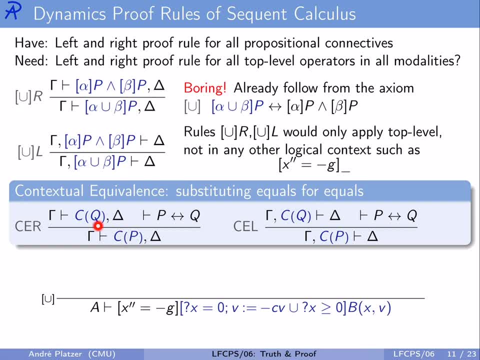 in this context, replace the occurrence of the formula P with the occurrence of the formula P by, instead, the formula Q. We can do that not just when P occurs in any arbitrary context in the right-hand side. we can also do the exact same thing when P occurs in any arbitrary 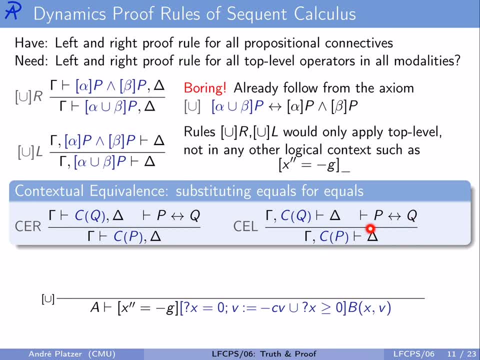 context in the left-hand side of the sequent. If P and Q are equivalent, then it doesn't matter whether we mention P or Q. This is really the intuitive principle of substituting equals for equals in the case of logical formulas, For example. here we can prove by the number: 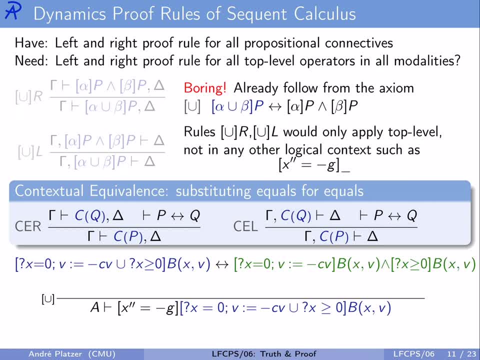 the non-diagnostic choice is the thing that's underlying it. By the non-diagnostic choice. this is equivalent to that, and because the blue formula which we've got here is equivalent to the green formula which we've got there, then of course it doesn't matter which one. 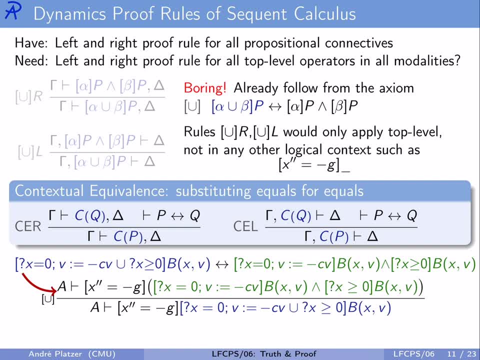 we mention So by the contextual equivalence principle. if we use this equivalence right here, we can write the green right-hand side instead of the left blue-hand side. Reminder: for this to be sound, it is, of course, super important to really have a proof. 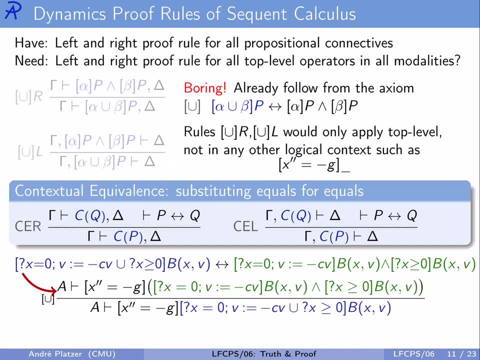 that P and Q are equivalent under no assumptions, Because in the middle of some logical formula context such as the right here, we have no way of knowing whether our assumptions are still true. But that's precisely what we've got from the axioms of differential linear. 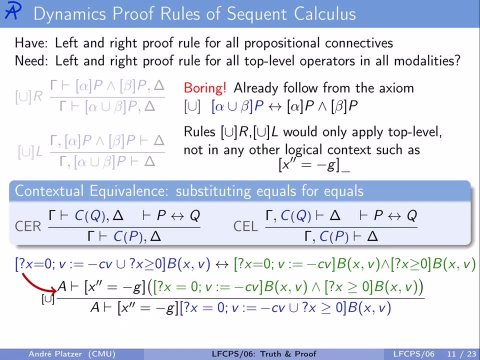 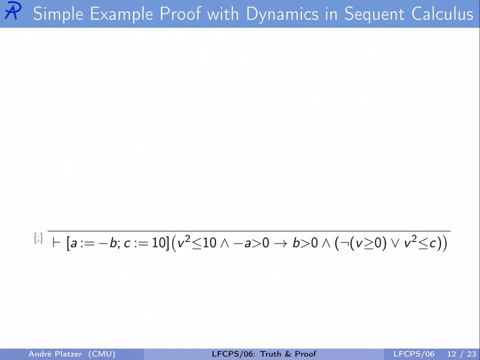 logic, Each of them is an equivalent, So let's make use of that. Here's an admittedly still super boring differential linear logic formula, but at least it's got some programs in it. So what we need to do here is use the sequential composition axiom. Yeah, we also have to use the contextual equivalence proof. 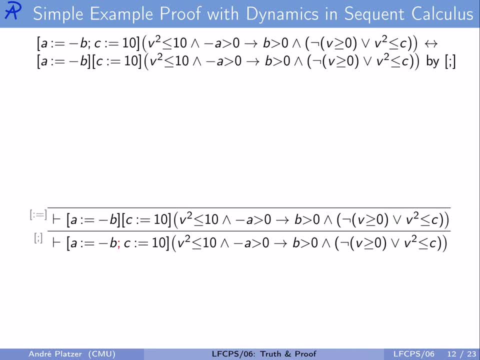 rule. but we usually just lighten the mention of that, Because this formula down here, here, here it goes, is equivalent to that formula up here, here it goes, by an instance of the sequential composition axiom. Of course it doesn't matter whether you mention the. 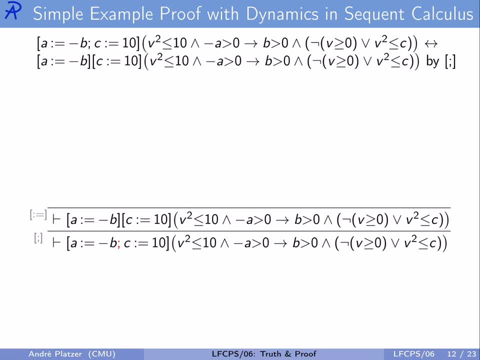 left-hand side or the right-hand side of this equivalence. It's looking very well. It replaced the left-hand side in any context- there's not a whole lot of context here- by the right-hand side. We will only say it was because of the sequential composition axiom. We wouldn't 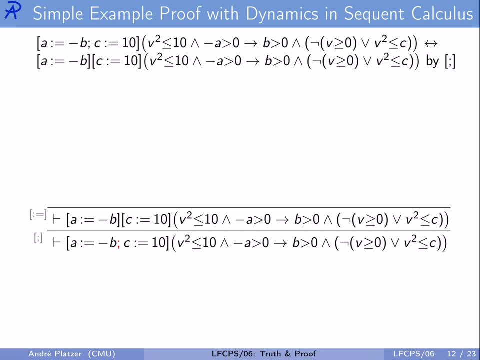 usually even write this down. Next, here we can handle the assignment axiom. This formula up here is equivalent to that formula down there. by an instance of the assignment axiom, Notice the occurrence of A. all of them in here are replaced by the right-hand side minus B. In this particular case we 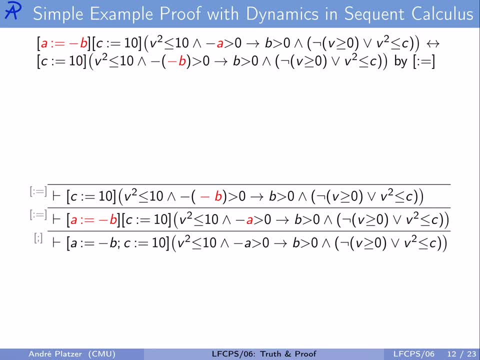 leave this assignment in here, but we could have worked in the other order. Just think about how you would do that. Then the only remaining modality is handled again by an assignment, where again by another instance of the assignment axiom. this formula here, by the assignment axiom is equivalent. 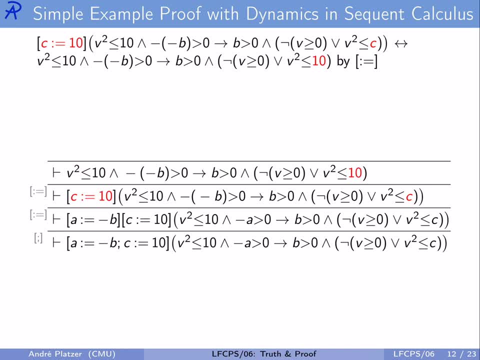 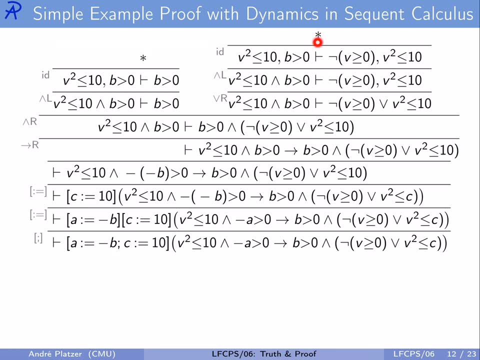 to that formula right there. It doesn't matter whether you mention the left-hand side or the right-hand side. Now we can simply copy-paste the proof we already had before, because, coincidentally, the remaining sequent that we have right here is equivalent to that formula down there. 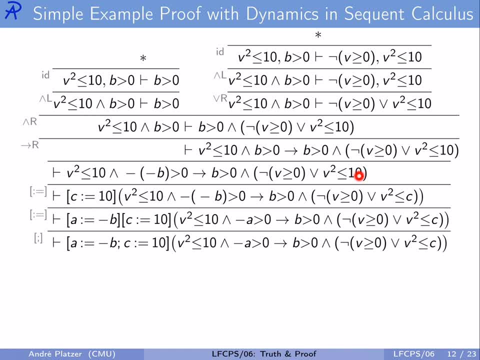 It doesn't matter whether we mention the left-hand side or the right-hand side. Now we can simply copy and paste the proof we already had before. But what we're simply doing is just the prepositional logic we already saw. Copy paste. 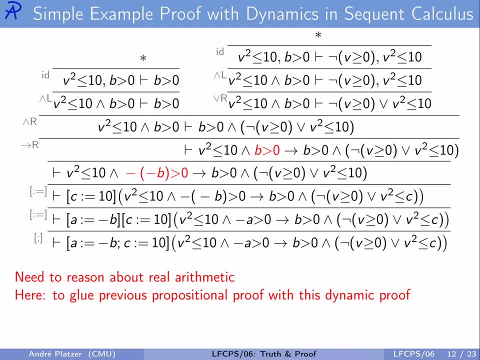 Slight twist Here and there. we don't quite have the exact same arithmetic form. In other words, we will also need to start to learn to reason about real arithmetics. But we already glued the previous prepositional proof with this little tiny bit of arithmetics together. 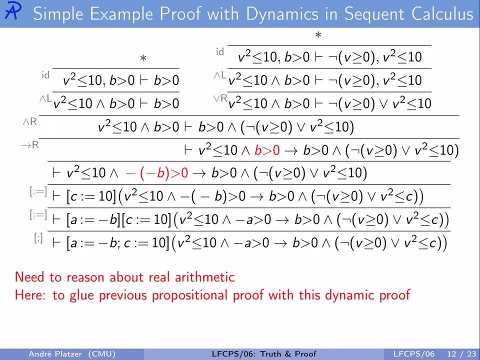 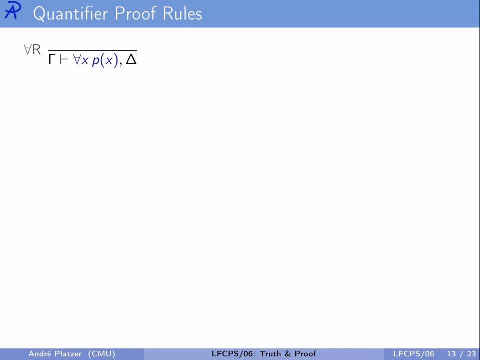 with the dynamics. proof that we have right here To have it perhaps not as time-consuming as we might like it to be, But we can simply Pretty rigorous proof of this differential, monotonic formula Good, We've seen proof rules for almost all the logical operators, for AND OR, implication and so on, but also 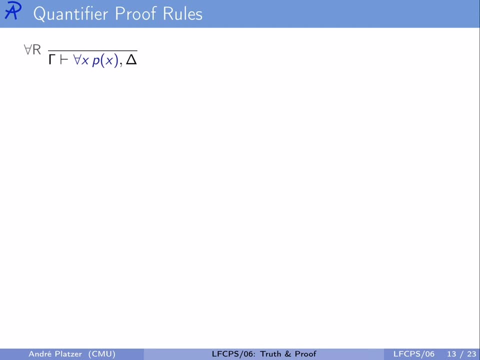 for the modalities box and diamond, for all the cases using the dynamic systems, axioms that we already saw last time, But we're still missing two. One of them is the universal quantifier, the other one the existential quantifier, But let's follow the same guiding. 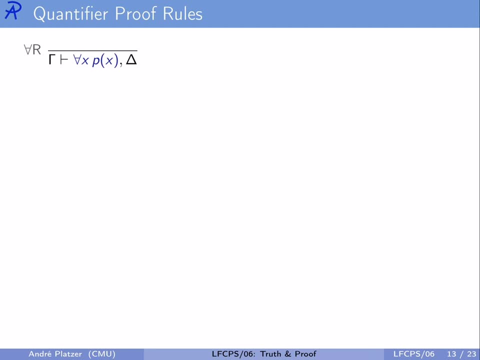 principle of designing them: A proof rule for the right-hand side occurrences and a proof rule for the left-hand side occurrences in a sequence. How would we go about proving for all x? p of x is true. Let's remember what we would do as mathematicians in order to 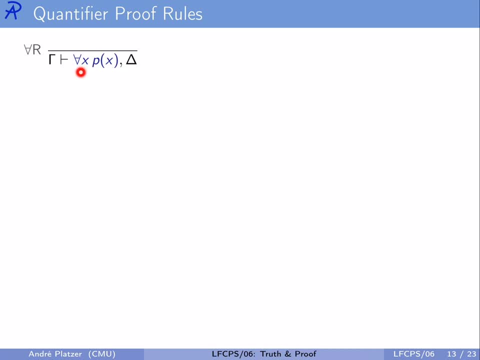 prove that p of x is true for all x's. we would just prove it for an arbitrary y and prove that p is true for y where y was really arbitrary. But we have to make sure that the variable y we choose to prove it for is really new. It's really arbitrary. That means, in particular: 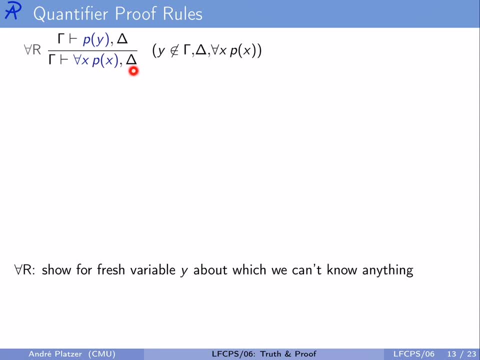 it cannot possibly occur in either gamma or delta or for all x, p of x, not free. at least We need to choose a fresh variable about which we cannot possibly know and silently assume anything because we've never used it before, For example, if you want to show that for 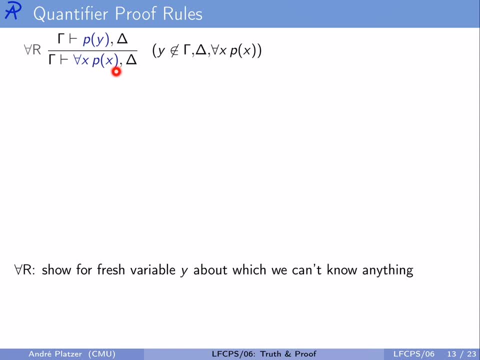 all x's x squared is greater or equal to 0, you would choose an arbitrary y and show that y squared is greater or equal to 0 and then walk back and say, yeah, but y was arbitrary, right. So of course that works for all x's as well, But it was important that y was arbitrary. 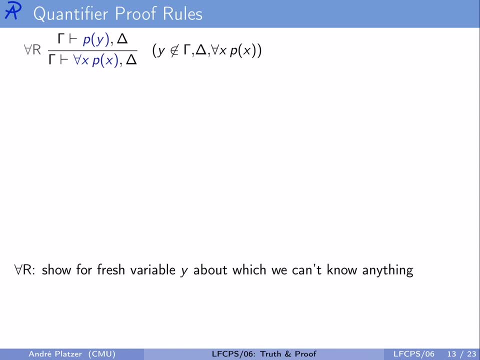 fresh variable about which we don't know anything. It's not sufficient to just prove it, for your favorite number is 0 and then walk away with the conjecture that it works for all of them. How would you prove an excess? Well, you would prove that there is a substantial quantifier on the right-hand side, that there 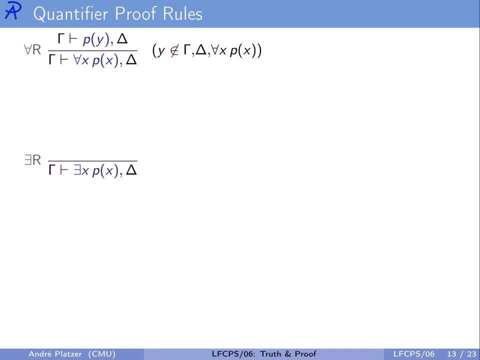 is an x such as p of x. Well, if we're trying to prove that there is an x such as p of x, we would just give the witness for the x that apparently exists, So some term, e which can mention anything at once, and prove that p is true of e. and because p is true of this, 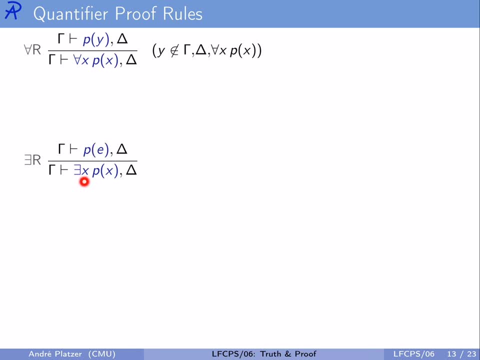 very term e. of course there is an x, So there is an x such as p of x it's called as e, but we just forgot about it, where this e can be an arbitrary term that serves as the witness. Imagine if you're trying to establish. 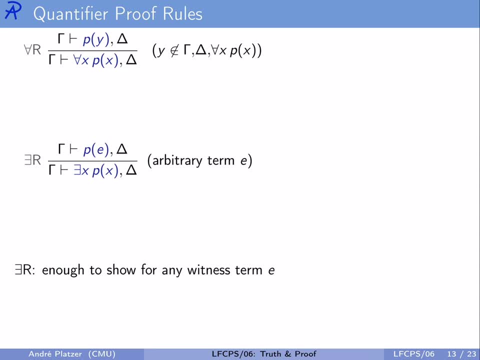 that there is a number whose cube is less than its square. the mathematician would choose a witness- 1 over 2, for example- and prove it for that. How do we know that there is an x such as p of x? Well, if you want to work with a universal quantifier in our assumptions, 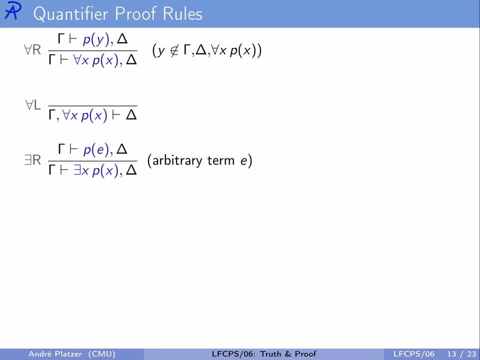 with the for all left proof rule. well, if somebody tells you among your assumptions you get to assume p of x for all x's, then I guess it's okay to also assume it for a very particular term, e- because after all, if we assume that p of x is true for all x's, 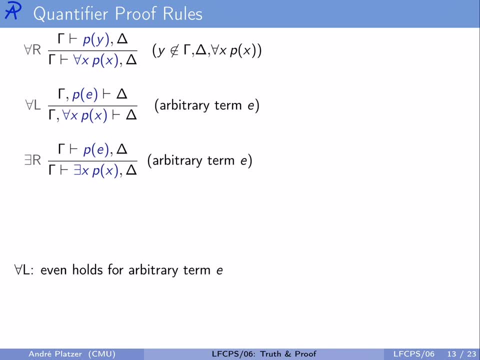 then it should definitely be true for the term e as well. that we made up arbitrary, All right. In other words, assumptions for all variable values also imply that we can assume them for one arbitrary one that we made up. How do we work with an existential quantifier? 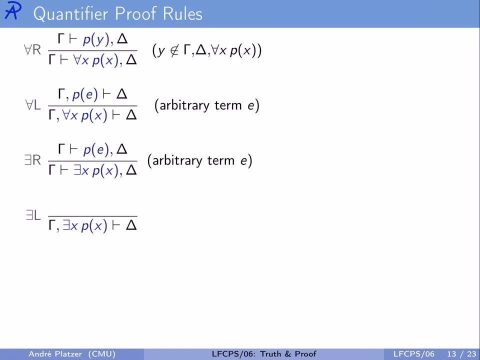 in our assumptions. If we assume, among other things, gamma, that there is an x for which p of x, well then we can assume that p holds for something, but we really don't know what it is. We really shouldn't assume anything specific about this something. In other words, we're 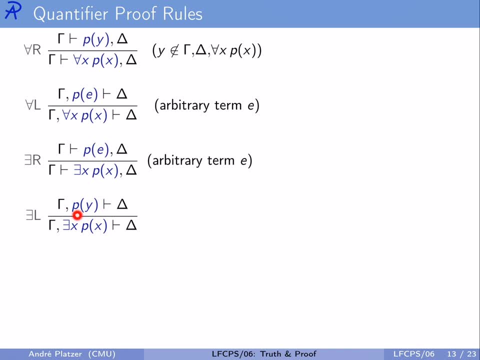 again in a situation where we can might as well assume that p is true of y, but it's got to be a fresh variable y that we haven't seen, or at least haven't seen free in what we've got here: gamma, delta, and there is an x p of x, Because, after all, if somebody 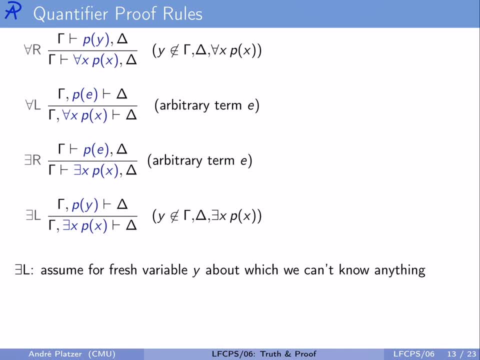 tells you: well, there is a number whose cube is less than its square, then you can't say, oh, okay, Let's do it. Let me assume that was 17, because it's not very true for 17.. But it's okay to say, let. 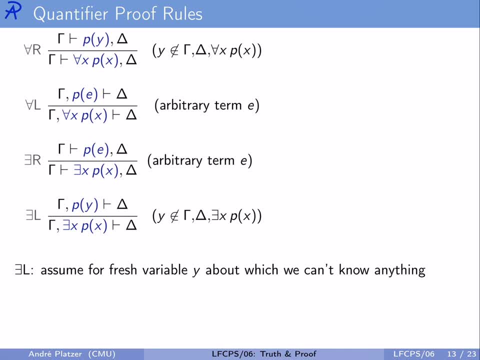 me call this number that apparently exists, whose cube is less than its square. I might as well call it y and work with this assumption about the y that I don't know anything about. This finishes up sequent calculus. proof rules, all of them. 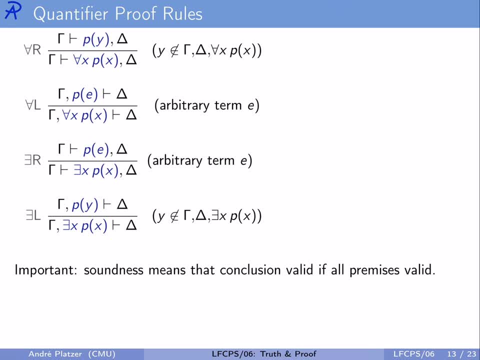 Notice for the quantifier proof rules. it was actually very important that soundness means that the conclusion is valid. if all the premises are valid, For example up here, it is important that it was valid, which implicitly says it's true in all the states, and that 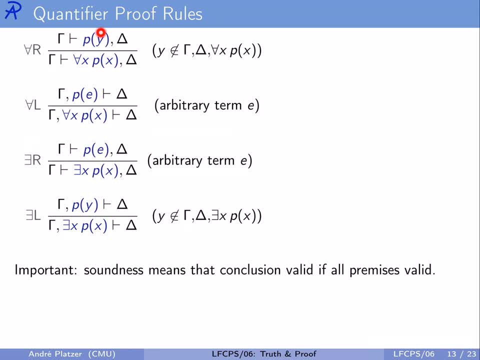 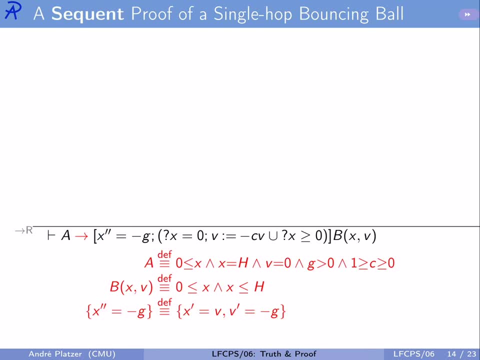 really actually already implicitly says it was true for all the values of the variable y, which is where the fall of x comes in as well. Let's use those sequent calculus proof rules for something good. Here's a bouncing ball In order to do a sequent calculus proof. well, we're trying to turn to a sequent and first. 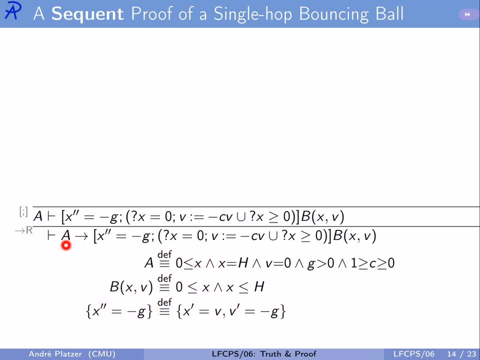 handle the implication by pushing the assumptions into our antecedent and proving the right hand side From now on. well, basically, the proof is the exact same thing that it was already in the previous lecture, when we were just working with dynamic systems, axioms, because 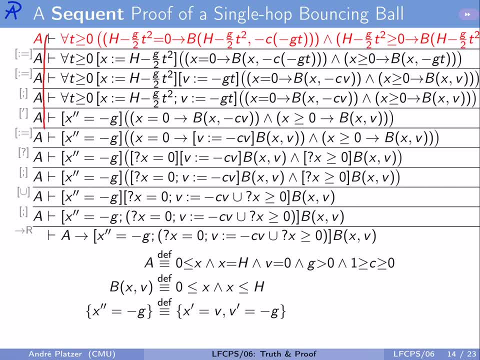 all we need to do is convert every time we mentioned implication into: well, now I guess we're in the middle of a sequent, but other than that, nothing. It really changes If we do this more carefully. Here we use an axiom to replace the left-hand side of an axiom by the right-hand side of. 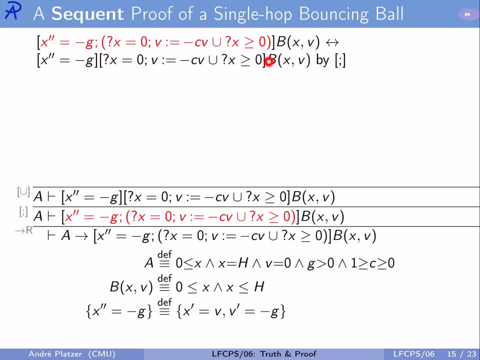 an axiom. The red is equivalent to this formula which occurs here. Then we use a choice axiom instance Again, now in the middle of it, this side is equivalent to that side, so we can also replace it in any context. Leave that alone. Here. then the sequential composition. 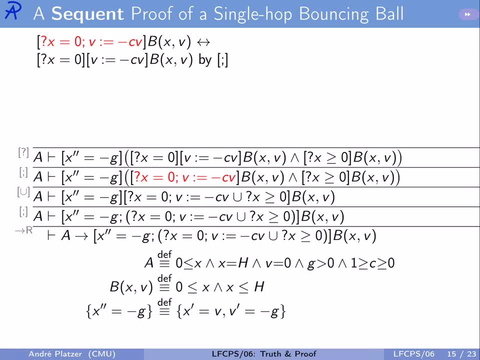 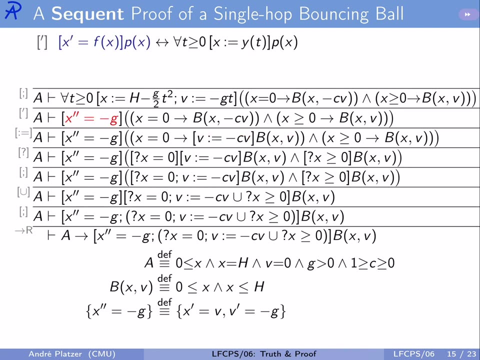 This is equivalent to that by the sequential composition axiom, so we can also write one for the other in any context. Here the tests are being handled, and now, finally, the differential equation is being handled. and now the resulting assignments here can be handled after first splitting the assignments in the sequential composition by an axiom instance, and then 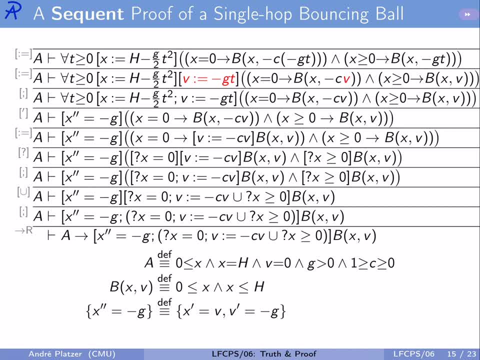 putting the assignments in, putting the values in, and so on. Now we're left with the exact same arithmetic that the bouncing ball already had before, and just observe that we were now following a structure of a proof more explicitly than we followed, almost incidentally, in the previous chapter. 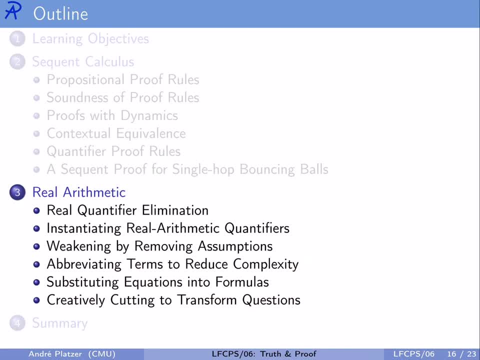 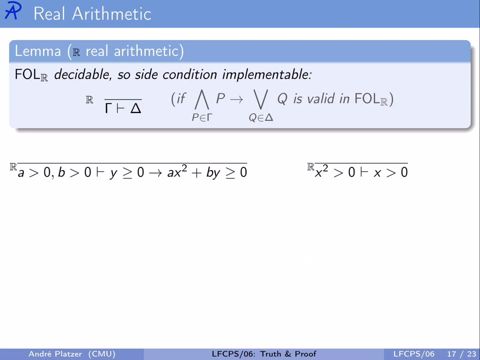 All of this structures the logical structure of the reasoning very well, but it doesn't tell us a whole lot yet about what we do with real arithmetic questions that come up. Let's give them a thought. For real arithmetic we're using a gigantic logical miracle by Alfred. 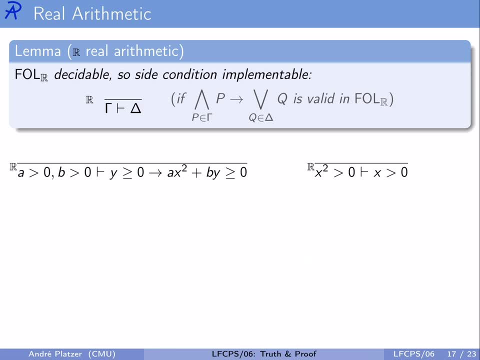 Tarski who almost a century ago proved that first of the logic of real arithmetic is decidable. So if we have a sequent with an antecedent gamma and a secant delta, and the formula here it is that the formula is the same as we have for the first and the second. So we have an antecedent. 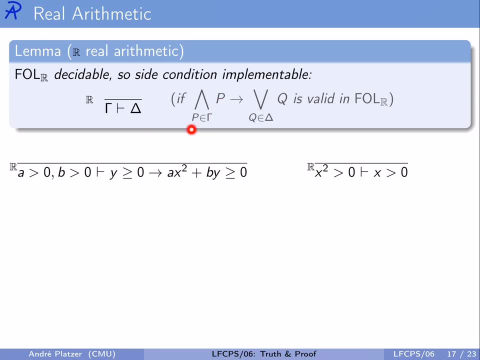 that this sequent represents. so conjunction of all the formulas on the left-hand side implies disjunction of all the formulas on the right-hand side If that formula here is first of all just the formula and first the logic of real arithmetic and also a valid 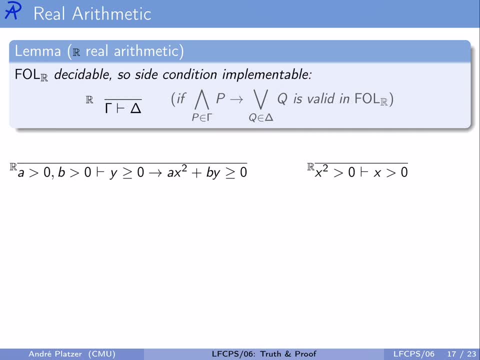 formula, so it is true in all the states. then we simply write down by real arithmetic. are we done with the proof? Of course, it is really important that the side condition that we have here really can be implemented. but it can be implemented by this miracle. 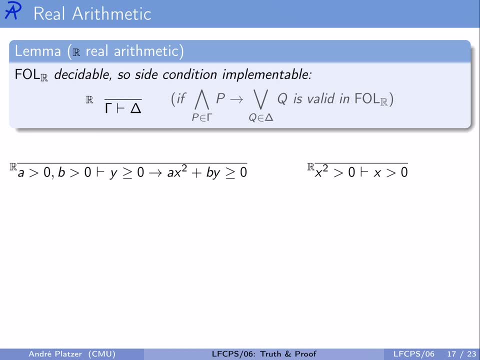 that Alfred Tarski came up with, that real arithmetic versus the logic is actually decidable. There's an algorithm for it, For example here: well, first of all, this is just arithmetic and second of all, it's a valid formula. So by real arithmetic we're done with the proof. 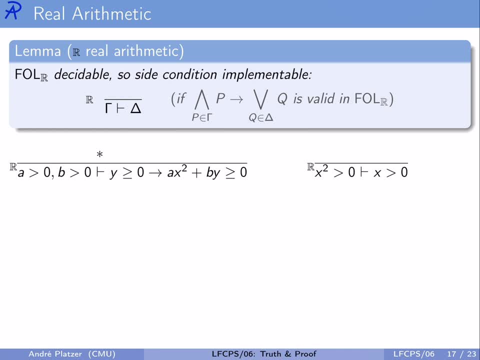 right here, Just like over here. This is just arithmetic, so we're done with the proof. No, no, no, no, no, no, That was too fast. That is actually not correct, because it is arithmetic all right, but it. 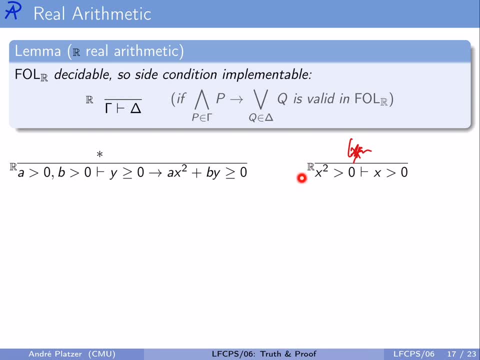 still has to be valid formula arithmetic, and this formula is not valid under all circumstances. just because if x squared greater than zero does not imply that x is greater than zero. just implies that x is greater than zero or x is less than zero. In other words this: 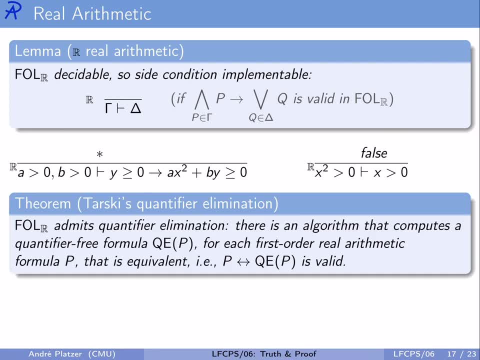 actually would be a false use of real arithmetic. Don't do it in the wrong way. The miracle here is that Tarski proved quantifier elimination. There is an algorithm that computes for every first of the logic formula P an equivalent formula that has no quantifiers, and the two are really. 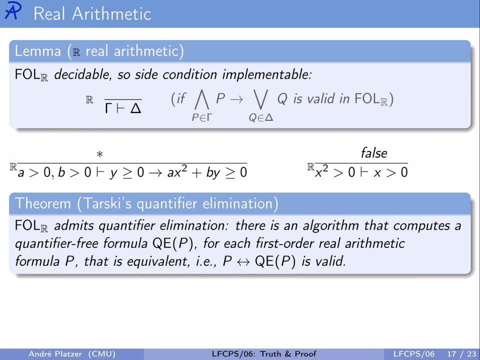 equivalent, meaning P is equivalent to QE of P is a valid formula under all circumstances and it doesn't even matter. That's it, Thank you. I'm glad that I didn't mention more variables free than it used to mention before. Yeah, 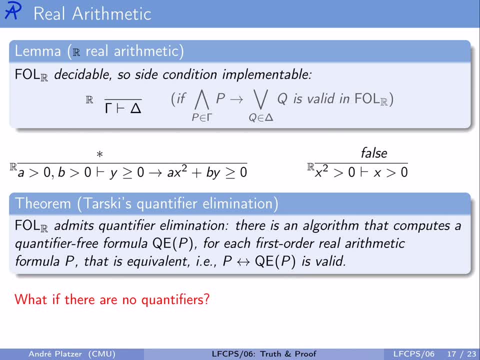 okay, That's cool, But what if there are no quantifiers Up here? there are none, so it's not completely clear how Tarski's quantifier elimination miracle applies, but it does, and here's the reason why: Because we can introduce the universal closure using an inverse. 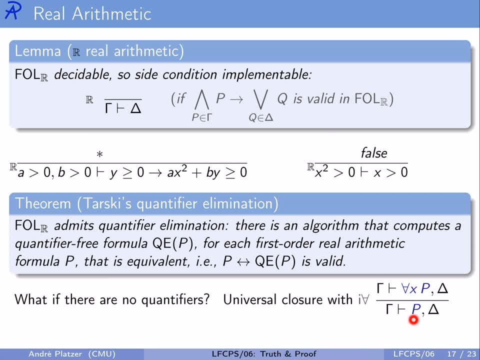 universal quantifier proof rule that basically just says one way of proving that P follows from a bunch of assumptions is to prove the more fancy statement that for all x, p is provable from the assumptions. Because sure, if we prove p for all x's, we also will have proved. 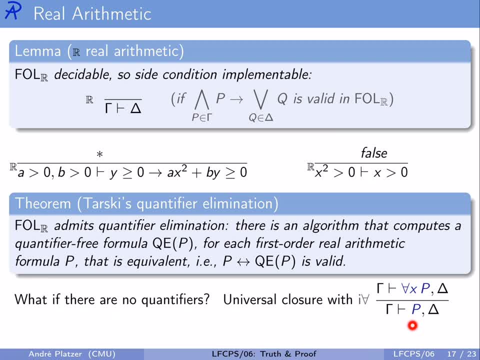 it for whatever particular variable x we had down here, possibly with some assumptions. So whenever we need to, we can dream up universal, not existential. but we dream up universal quantifiers because, if anything, it makes the proof harder, not easier. 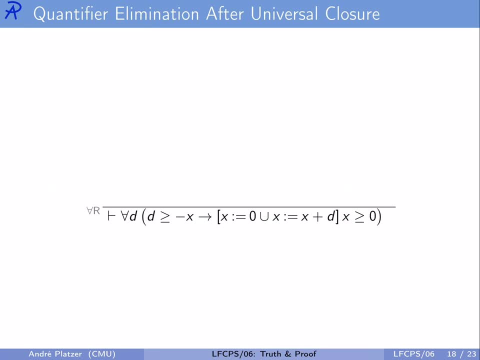 For example here, in this circumstance, here we've got a universal quantifier, so maybe you could think that you should use quantifier elimination for the job. but that's not the case, because it's not really first of the logic of real arithmetic that we have here. 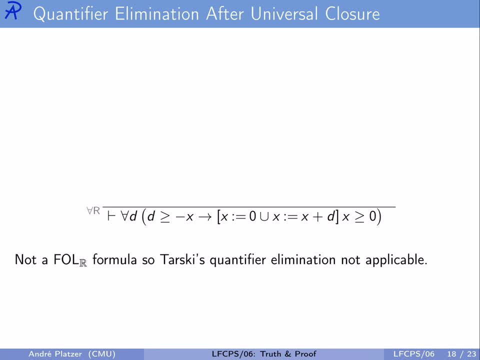 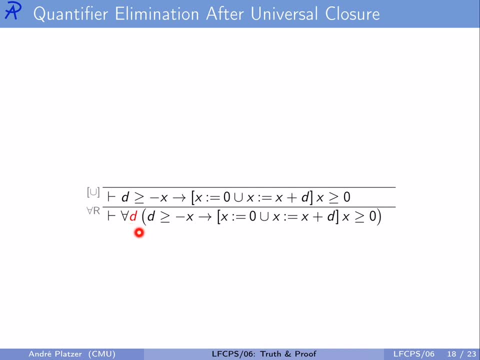 x, So we can prove a universal quantifier. We do that by just dreaming up an arbitrary value- We can still call it t, because we have no assumptions about t here- and prove it for this arbitrary value. Then we can, for example, work on the choice with the axiom of non-deterministic. 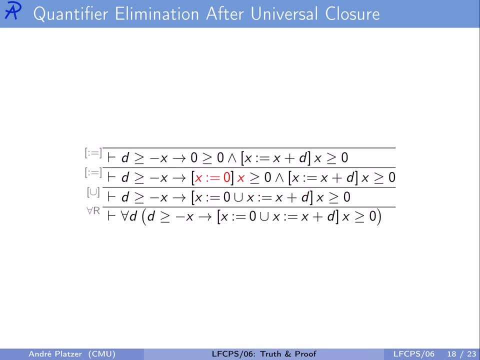 choice. Then work on the assignments here and work on the average assignment there, And now we've got real arithmetic. If we're strict about it- for example, if we're not- Tarski can eliminate quantifiers. We have got none, but we can introduce them again. 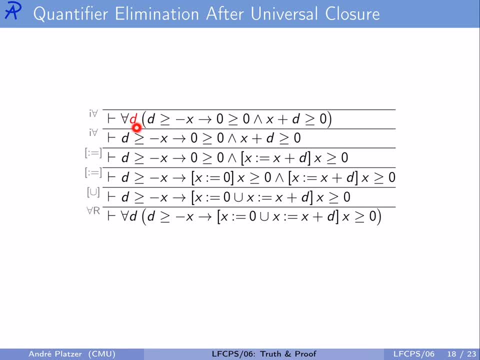 By the inverse quantifier rule, we can dream up a universal quantifier for d. Well, we can also dream up a universal quantifier for x, which was never there before. Now we have a formula where every variable is quantified, Because Alfred Tarski can perform quantitative. 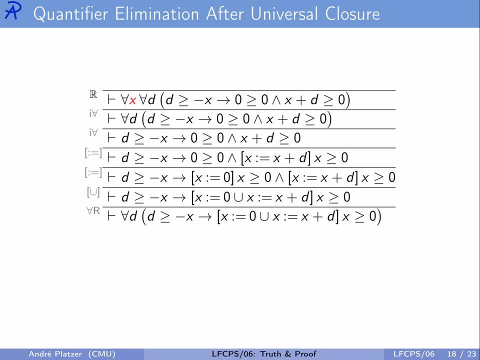 elimination on this and give us back a logical formula that's equivalent, but with no additional variables. it means that the only formulas that Arthur Tarski could be handing back to us are the ones that don't mention any variables. If they don't mention any variables, all we 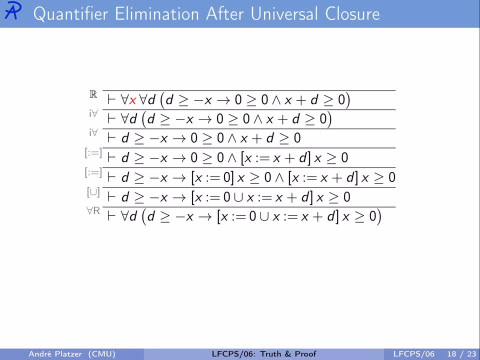 need to do is evaluate things like whether 7 is greater than 0 and stuff like that, which means we will be able to find out whether that formula is true or false, because it cannot depend on the state anymore. In this case, it is actually true, so we will be able. 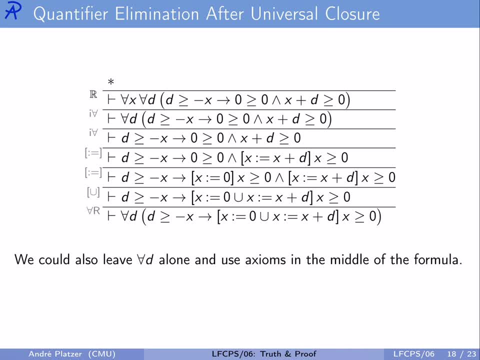 to prove that just by real arithmetic Notice we could actually do that We actually also have just left the poor for all d alone. just work in the middle of it right away, and then we spare ourselves the detail of having to reintroduce this new universal. 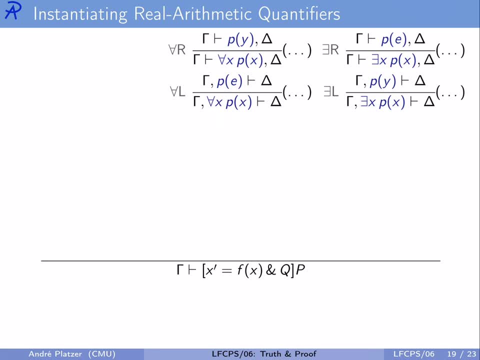 quantifiers. Now, real arithmetic decidability is a big miracle of logic, but its complexity of the algorithms that decide it isn't amazing. In other words, oftentimes it can be very important to simplify and learn. In other words, when you're thinking about simple logic, the arithmetic questions before, 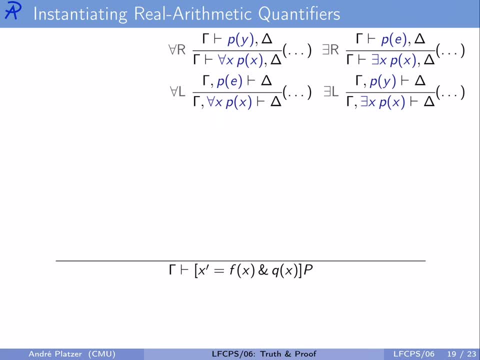 you proceed. One of the techniques to logically simplify real arithmetic questions will simultaneously enable us to practice quantifiers and learn something useful about differential equations, Namely when we're giving a question about a differential equation, x prime equals f of x within the evolution domain constrained q of x. does the postcondition p hold afterwards? 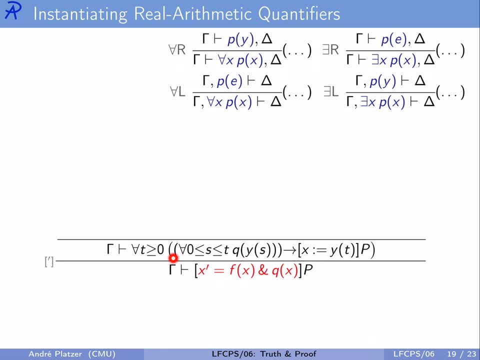 In order to prove that we can solve the differential equation using the solution axiom, which will enable us to work on a universal quantifier By the for all right proof rule. we prove a property for all times t by proving it for any arbitrary time t, assuming we haven't used t here. 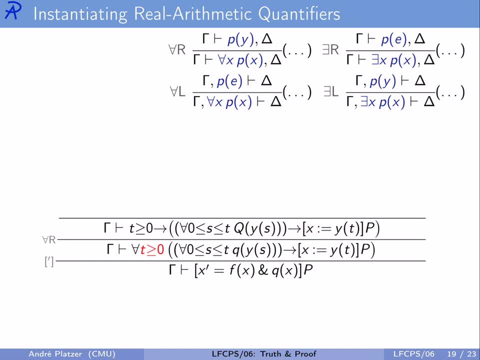 Then we can use the implication proof rule to assume the left-hand side t greater or equal to 0, to prove the right-hand side. Then we can again use the implication right proof rule to move this assumption on the assumption stack as well. Now we have an assumption for all intermediate times s between 0 and t. 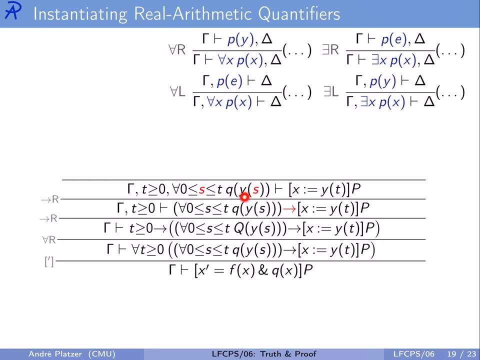 Is the evolution domain constraint Q true for the value that that t is The solution Y has at this intermediate point in time? S? Of course, one thing we can do with it is use the for all left proof rule to instantiate this intermediate point quantifier. 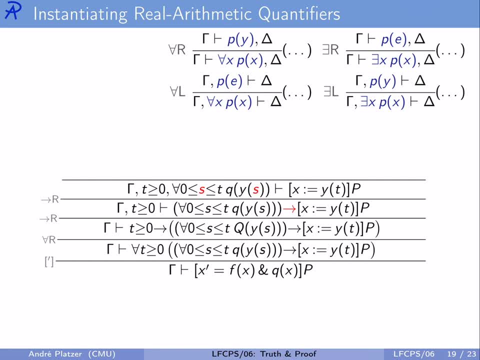 for some helpful time. What do you think is the most interesting point in time where the evolution domain constraint is true? The one we're at right now. We're currently at time t, so that's the most fascinating one to be able to learn something. 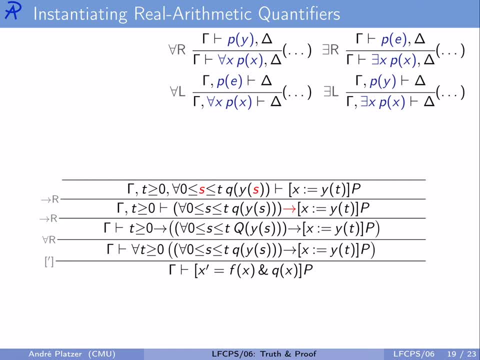 about The evolution domain constraint is true at that moment. so let's insert the concrete time t that we're interested in for S wherever there used to be S, now there's t. Then work with the implies left proof rule to prove the left-hand side of this implication. 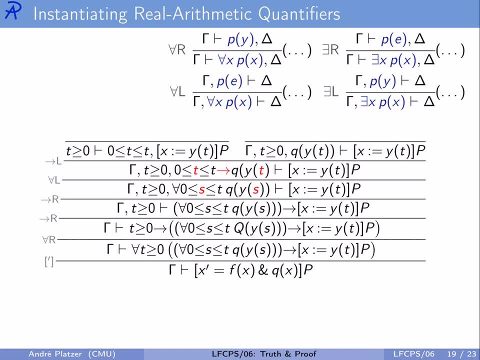 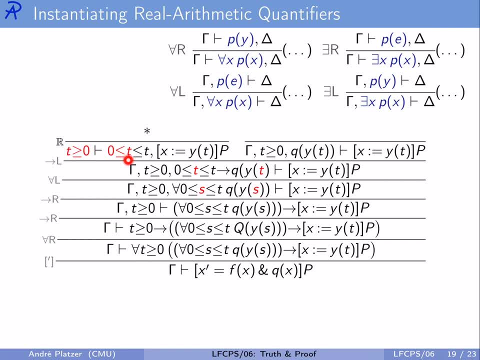 t greater or equal to 0. So proving that this is true is actually very easy, because, well, we are already assuming t greater or equal to 0. Proving its conjunction that 0 is less or equal t is easy, And proving the other conjunction implicit here, that t is less or equal t, is also easy. 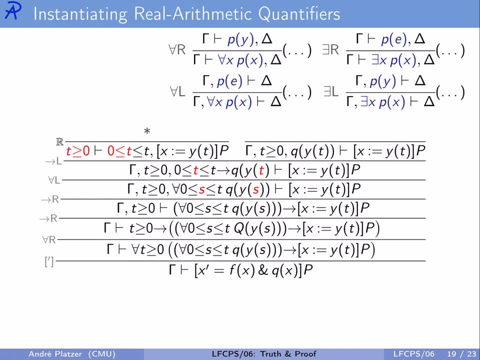 just by trivial reflexivity arithmetic. That leaves us with only the left-hand side to worry about. Of course, without knowing more about what gamma and q and p and y are, we cannot possibly succeed with a proof of that. But we walk away with the insight that this proof could always be done if we have a solution. 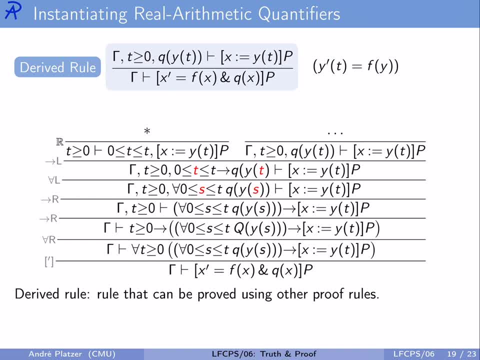 so we summarize it with a derived proof rule that says: if we would like to prove this, we might as well prove the only one remaining question, namely that one up here, Of course under the usual assumptions for solutions, namely that y actually is a solution. 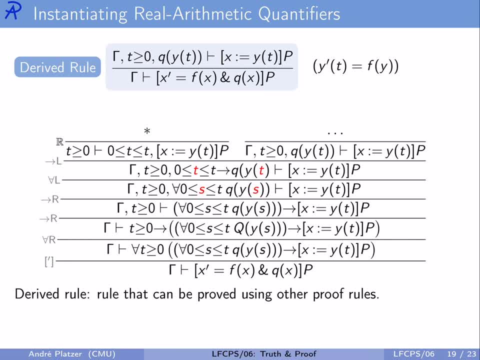 of a differential equation and starts from the appropriate symbolic initial value, and t is a new time variable and all that sort of thing. But this now is a different style of justifying why a proof rule is important. It's not one that we have to bake in and convince ourselves with the semantics that it is right. 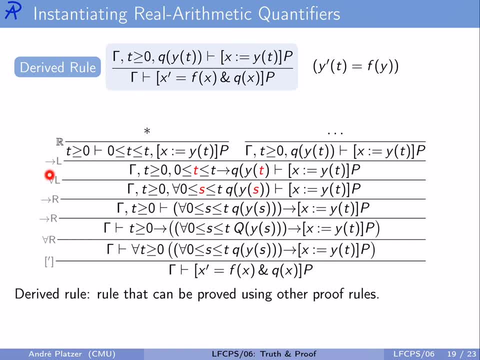 It is a proof rule that we simply read off by mixing and matching other proof rules and axioms together in order to succinctly summarize what we've learned this way around. Now, when we look at the remaining derived proof rule, it tells us that if we're trying 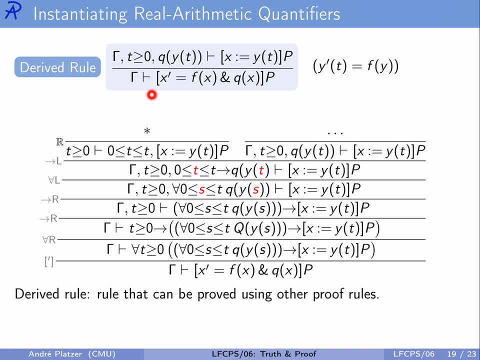 to prove a box property of a differential equation with an evolution domain constraint q, And of course the evolution domain constraint actually has to hold at all the moments in time. but it is okay for a proof to merely work from the assumption that the evolution 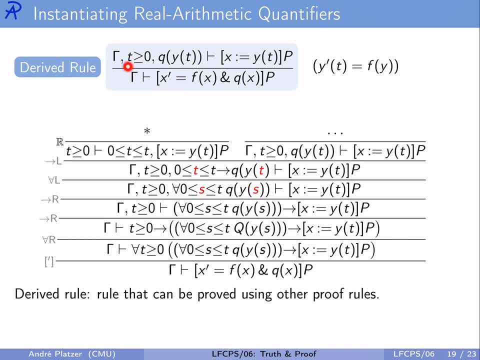 domain. constraint q is true at the end time t, that is arbitrary, when that suffices in order to prove the postcondition. And yeah, this instantiation that we did down here of a quantifier actually is helpful because it saves work for the real arithmetic quantifier elimination because, hey, we eliminated it. 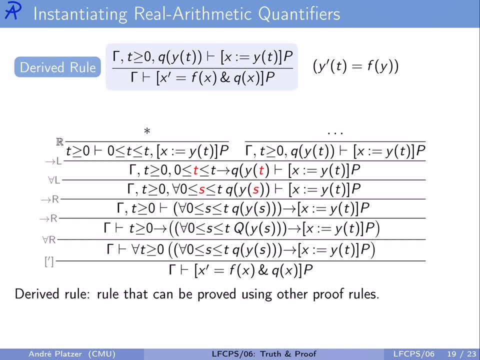 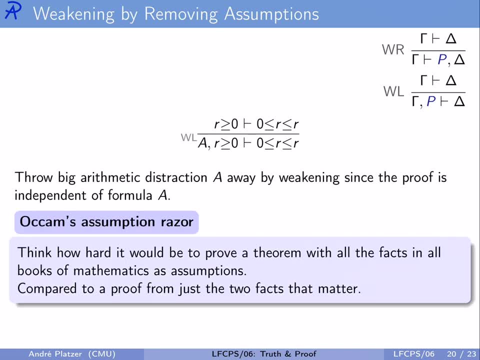 by instantiating it appropriately. So this can be a very helpful idea in your proofs to manage proof complexity of real arithmetic as well. Another thing that can go wrong in arithmetic is that you have a ton of stupid assumptions. Some of them are very clever even, but the arithmetic question you have is just like: 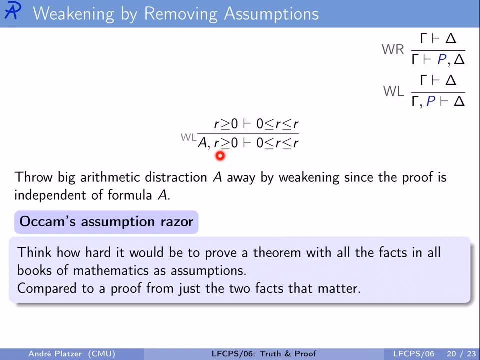 in the case, If you saw a moment ago a very easy one- from the assumption that r is greater or equal to 0, it's pretty easy to prove that 0 is less or equal to r. oh, and also r is less. 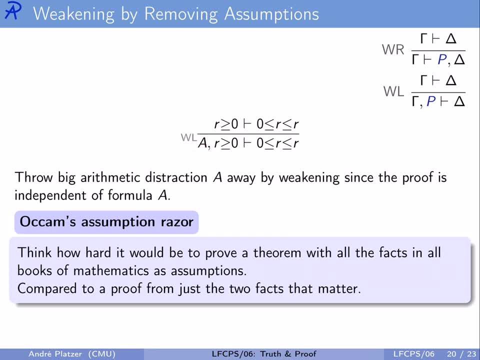 or equal to r, which has nothing much to do with anything at all, with the additional assumptions a that you have available. Remember, your proof in sequent calculus is carefully managing exactly the set of assumptions that you have available. It's not telling you which of them are useful. 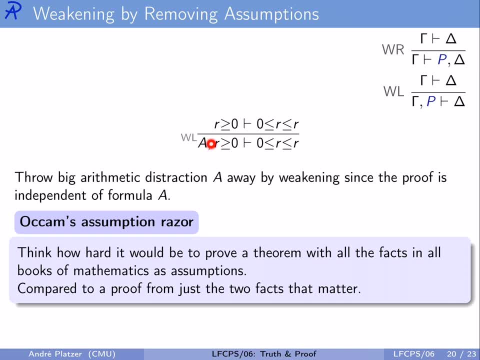 If you have a very complicated arithmetic question. it's not telling you which of them are useful. It's not telling you which of them are useful If you have a very complicated formula. that can be a big distraction to the real arithmetic decision procedure. 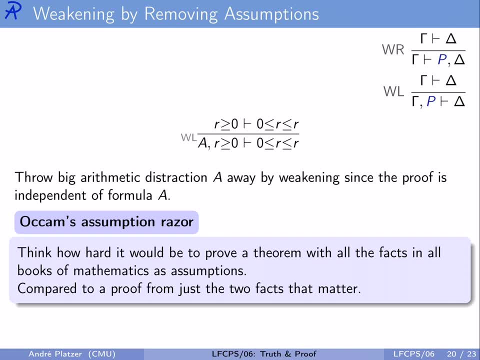 This is essentially Occam's Assumption Razor. Think of it: how hard it would be to prove a theorem if you have all the facts and all the books of mathematics available as your assumptions. It's going to be a gigantic implication, with lots of assumptions and they're not helpful. 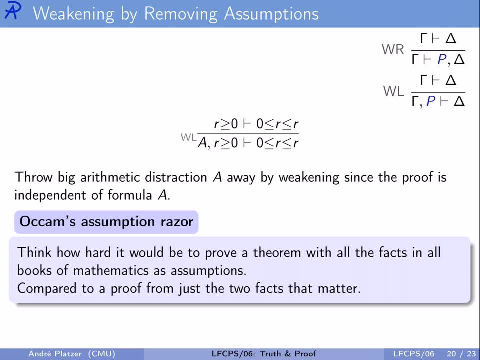 compared to trying to do a proof if somebody gives you just the two facts that actually matter for your argument. So, by using your intuition, you're going to be able to prove a theorem. You're going to be able to prove a proof if somebody gives you just the two facts that 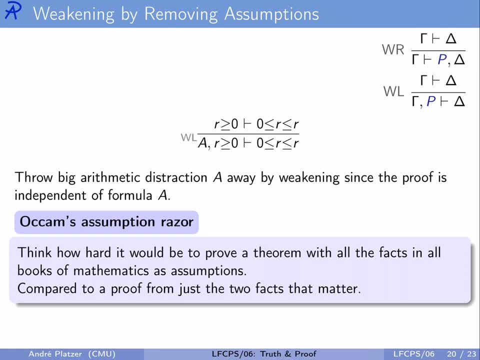 actually matter for your argument. You're going to be able to prove a proof if somebody gives you just the two facts that actually matter for your argument. You can make the arithmetic a lot more scalable by deleting assumptions, which is always okay- by the weakening left proof rule, the one that says: in order to prove that from the 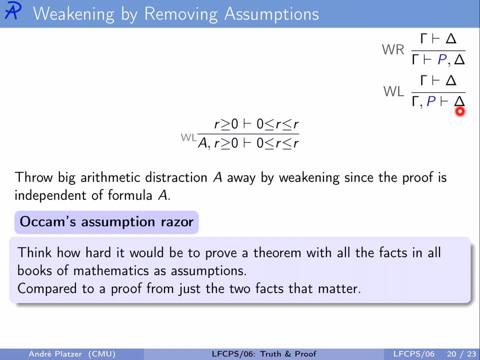 assumptions gamma as well as p delta follows. it suffices to prove that already just from the assumptions gamma does delta follow. It's okay to delete assumptions. It's just not a great idea to dream them up, because that would be unsound. 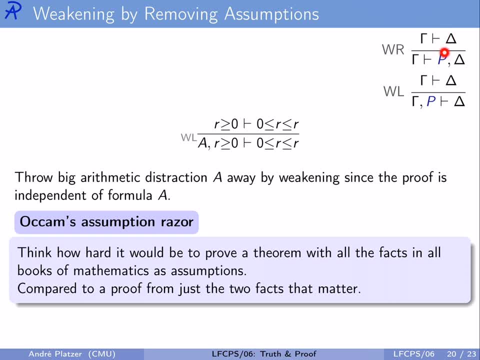 with the weakening right proof rule? is it okay to delete alternatives that we are trying to establish on the right-hand side? The thing on the top is always a bit harder to prove than the things on the bottom, But here it's actually easier computationally, even if magically. 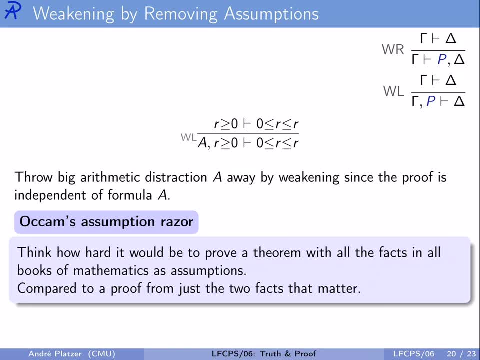 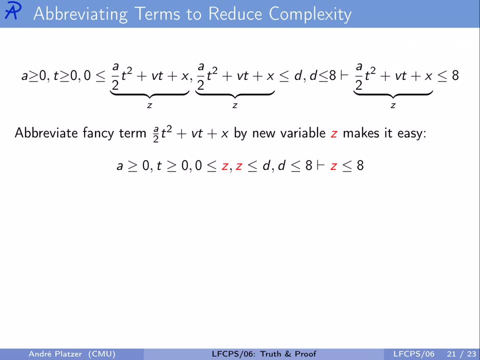 we made, assumptions disappear, which makes it seemingly harder. It's computationally a lot easier. Another thing we can do to help arithmetic along is abbreviate terms to reduce the complexity. Here's some arithmetic, and while it may or may not be true, it's hard. 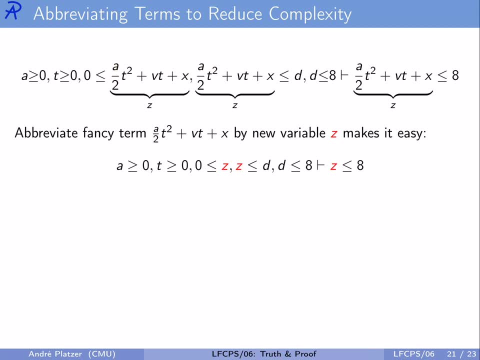 to see. but notice here the exact same fancy, complicated term is appearing a bunch of times. If we simply call this term z, give it a new variable name, then the remaining arithmetic is just that. We've got some arithmetic distractions, but it is already easier because all that 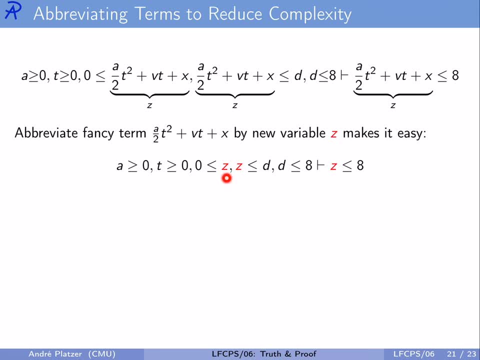 we are asked to do now is, from the assumption that zero is less or equal z and z is less or equal v and d is less or equal eight, to prove by transitivity That z is less or equal eight, which is comparably easy. It can be very easy for arithmetic. 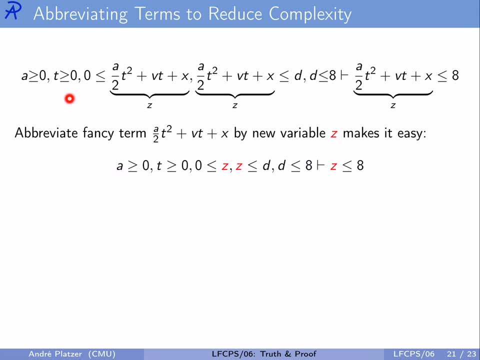 procedures to see if it is present, like so, and very hard if it is hidden behind very complicated arithmetic expressions. instead, We will not now develop a proper proof rule for introducing sensory abbreviations, even if you're already welcome to use them in your proofs, because that will be a topic of a later chapter, 12 to be precise. 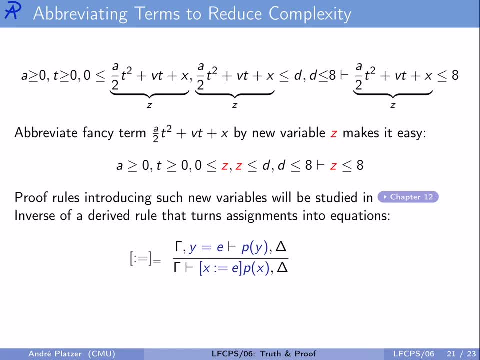 But in order to just give you a hint of how this works, this actually inverse of a derived proof rule that also is useful, one that turns assignments into equations. There's another way of handling: that we assign that value of the term e to the variable x and prove: 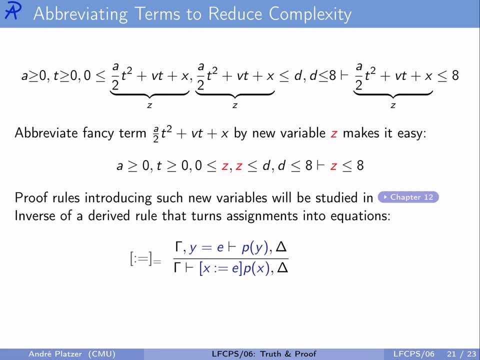 that p is true of x is to assume the equation that y is equal to e and then instead prove that p is true of y Where? Because for soundness reasons it is extremely important that y again is actually a new variable. Just think of how awkward it would be if our assignment here would be x assign. 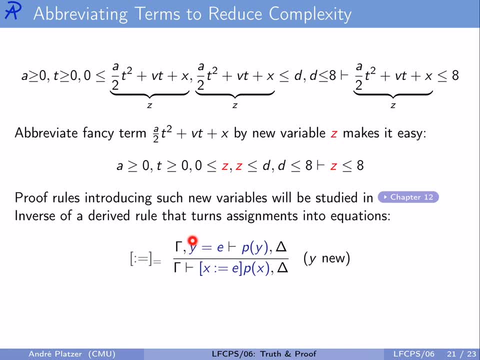 x plus 1, and then we would have as our assumptions x equals x plus 1, which is really impossible of an assumption. But if y is a fresh variable, basically denoting the new or static single assignment form value for the variable x, then it's sufficient to prove that p is true. 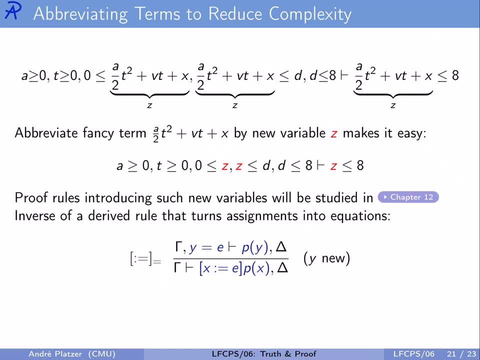 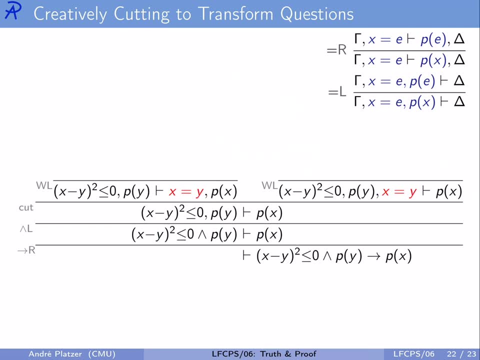 of y. This can sometimes be useful, but it's already derived. Another thing you can do to simplify arithmetic is to use a creative cut, So a cut like Gerhard Gentzen. prove a lemma and then use a lemma, but you use it in a clever way to dream up arithmetic that simplifies. 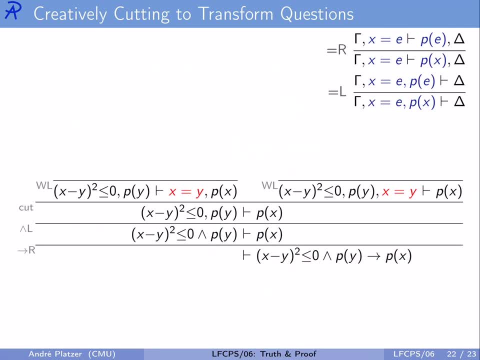 your questions. Think of it this way: If you're trying to prove this ordinary propositional logic, proof rules, turn it into that question. and now you have among your assumptions that x minus y is true of y. P is equal to x, square is less than or equal to zero, and some big and fancy formula P of. 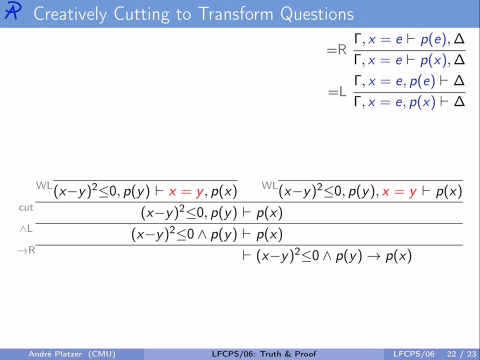 y and a big and fancy formula P of x that you're trying to prove from that. Now, that can be hard, but a clever arithmetic insight would lead you to observe that- wait a minute. if x minus y square is less than or equal to zero, then of course x has to be equal. 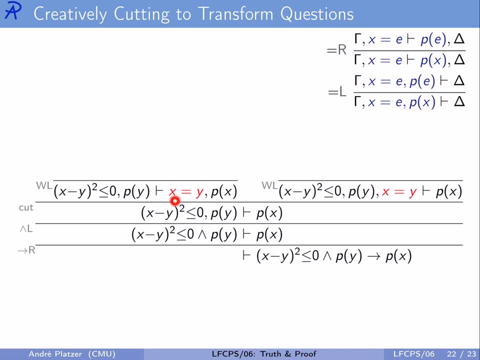 to y. So you prove with the cut the lemma that x is equal to y and then assume the that x is equals y in the rest of the proof. How you do the left-hand side premise is by deleting all the arithmetic distractions that are not of significance of the proof. First, 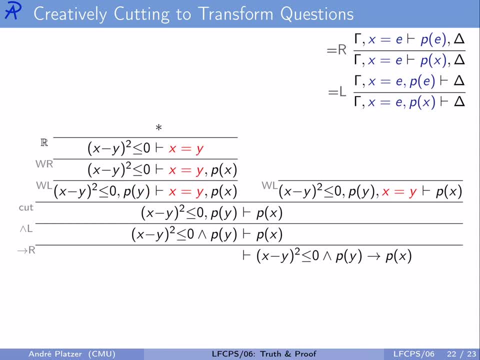 that is a question that's irrelevant of what the assumption P of y is, so let's delete it away. There's also a question that's irrelevant of what the other alternatives P of x is on the right-hand side. All of a sudden, this arithmetic is a piece of cake, to prove by: 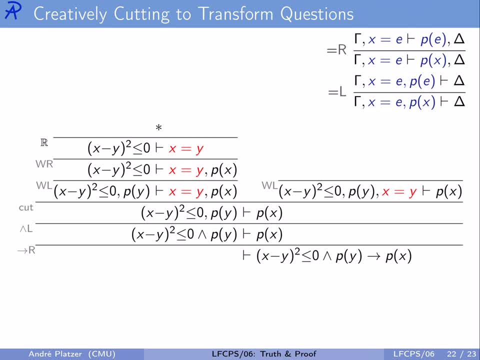 decision procedure. But now we've established that x equals y is an okay assumption to be using. Now we delete away the higher degree assumption- x minus y squared is less or equal 1, to just have P of y together with x equals y. From that we're trying to prove that P 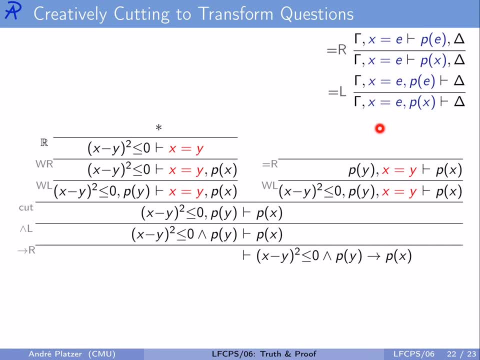 is true of x. Now we have proof rules for handling equations, For example the one that says if we have x equals e among our assumptions on the left-hand side, then we're going to have P of x. Then proving P of x can be reduced to instead proving P of the right-hand side. 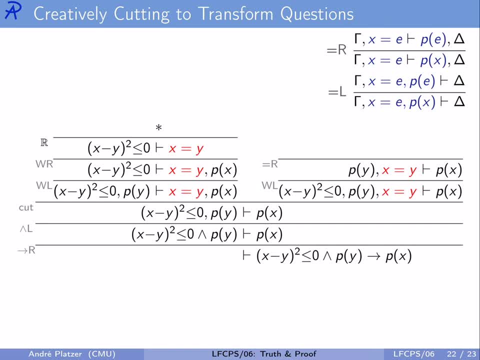 e. Sure, if they're assumed to be equal, we can replace equals with equals, Likewise if that replacement has to be done on the left-hand side in the antecedent. So here we'll use the equality of right proof rule to say: well, but since we do assume 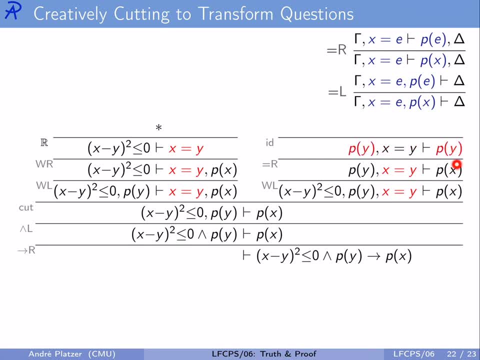 that x is equal to y. it doesn't matter whether we say P of x here or P of y here. All of a sudden, the identity proof rule is able to do that, which is of course much easier than having to ask a multiple of x. 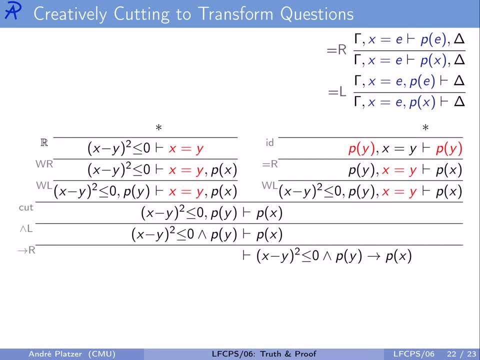 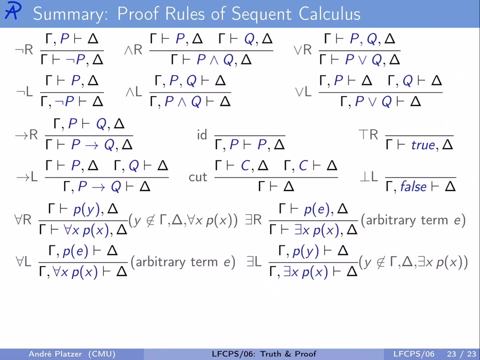 Now let's see how we can monitor arithmetic decision procedure for the job. Notice: this arithmetic simplification hinged on the fact that we observe something clever that we prove first and then assume. from that point forward, We can get arithmetic distractions out of the way. Let's summarize what we've learned in this chapter. We've seen proof. rules for 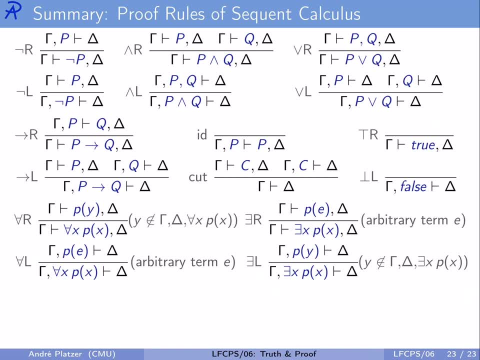 sequent calculus that have a proof rule, left-hand side For the right proof rules. in the succident these are proof rules for proving that a formula of this particular shape is true, For example P and Q. we prove by proving that P is true. 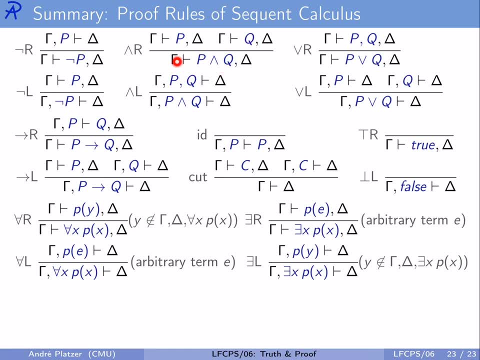 and separately proving that Q is true. even if we have the exact same assumptions, gamma is still available. and even if we have the exact same alternatives, delta is still available. There's also a proof rule for each of the operators, For their occurrence on the left-hand side, For example. again, if among our assumptions 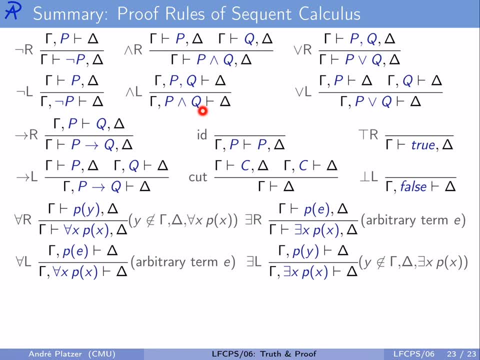 we find P and Q. well then we can proceed with a proof by just splitting the conjunction into two separate assumptions and assume the old assumptions gamma, together with just the left conjunct P and the right conjunct Q, because that's sufficient. All of these are actually very easy logical operations With a bit of attention for the 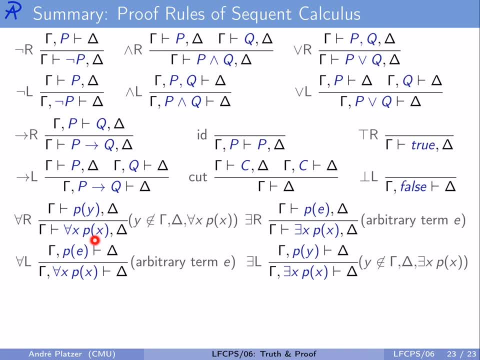 quantifier. we'll get to that later. There are proof rules. For example, I'm going to prove that for all x, P of x, we have to actually dream up a new variable, y that didn't occur free in what we had before and prove. 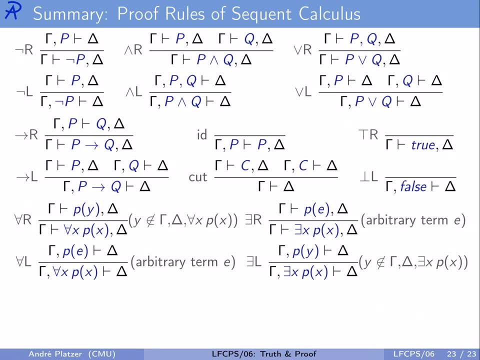 it with this new arbitrary y that P is true of y. The only slightly different proof rule is the one for real arithmetic, which says: well, we were just left with real arithmetic and that formula that this sequent corresponds to. a conjunction of left-hand side implies.